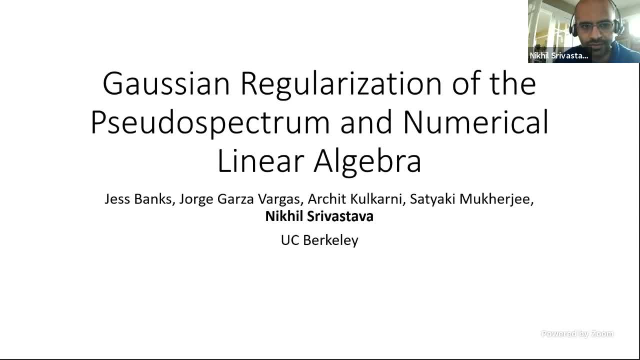 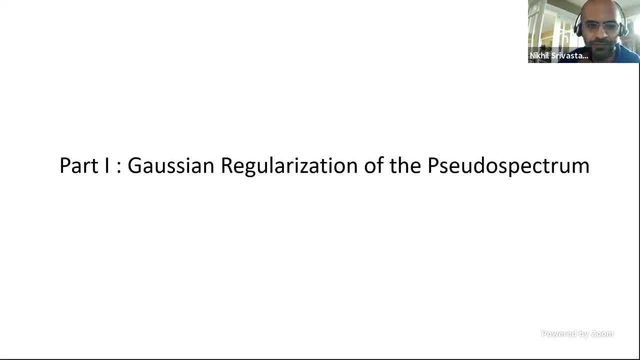 talk. I'll talk about an application to numerical linear algebra. OK, so part one. So, and please stop me if you have any questions- So the proofs that I'm going to present are very simple. They're among the shortest proofs that I've ever talked about, So I hope that you can. 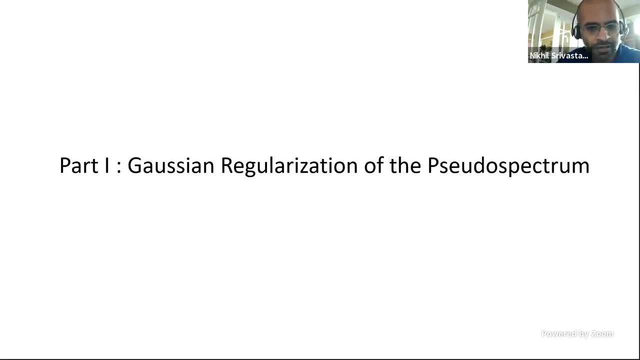 understand all the details And please stop me if you have questions. OK, so the talk is about diagonalization. OK, so what is that? So a matrix, a complex square matrix, is diagonalizable if it's similar to a diagonal matrix. 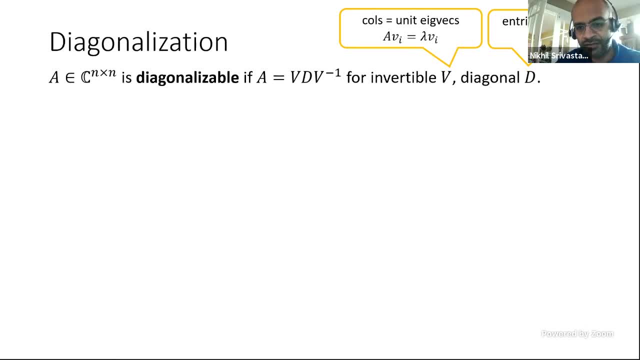 So you're going to get A as V, dV inverse, where V is invertible and D is diagonal, And if you do this, then the columns of V contain the right eigenvectors of A and then the diagonal entries contain the eigenvalues, which are some complex numbers. So here's a matrix that's diagonalizable. S. 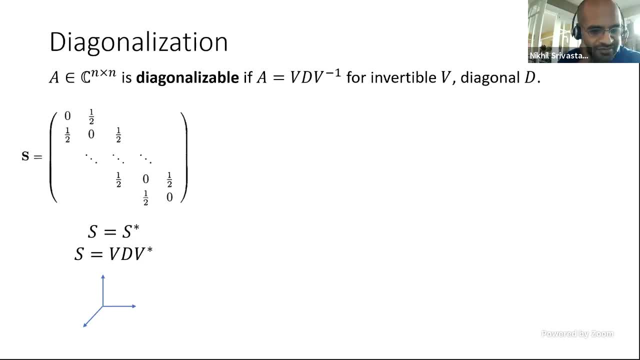 So this is a symmetric matrix. So OK, it's Hermitian, It's equal to its adjoint And, as a result, it's actually orthogonally diagonalizable. So there's an orthogonal matrix. So it's a matrix that's orthogonal. So it's a matrix that's orthogonal. 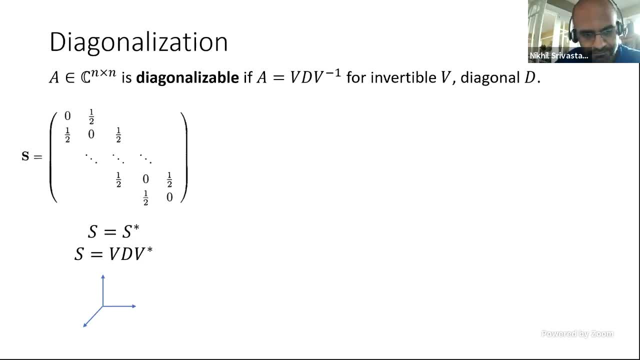 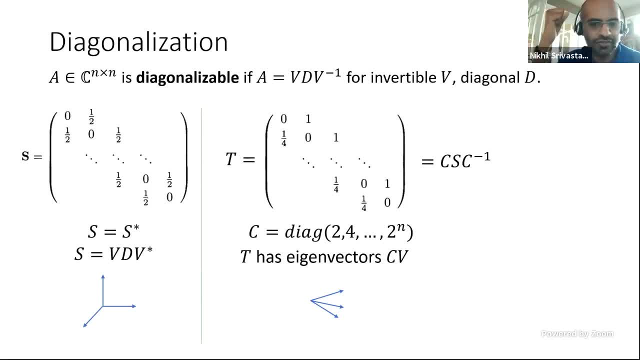 are exponentially increasing. So T looks superficially quite similar to S, except that it's not Hermitian. And because it's similar it has the same eigenvalues. but its eigenvectors are now given by Cv and they're highly non-orthogonal. So this is one of the key. 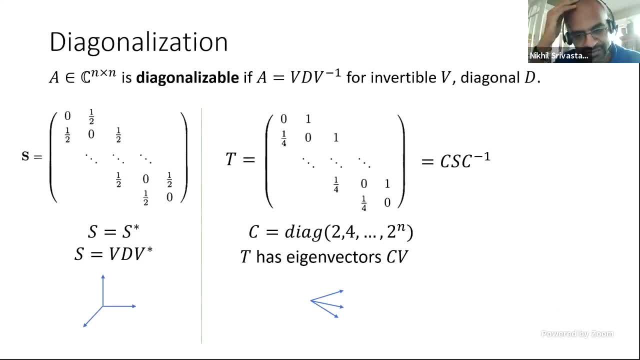 differences between Hermitian and non-Hermitian matrices, that the eigenvectors in this case are linearly independent but not orthogonal anymore. So this is also diagonalizable. And then here's a matrix that's not diagonalizable: the Jordan block. So 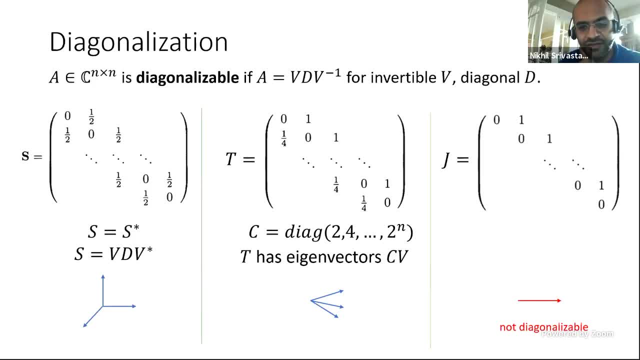 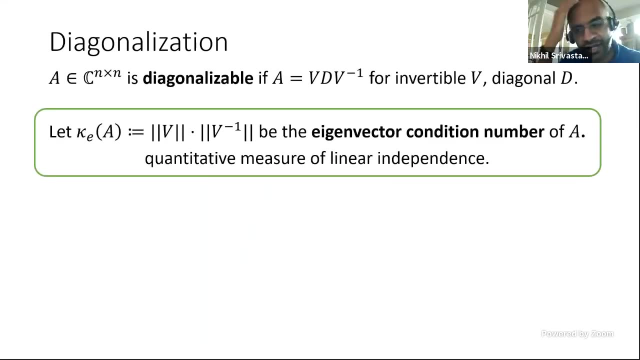 okay, this only has one eigenvector. it does not even have a basis of linearly independence. So the question I want to study in this talk is related to quantitative diagonalizability. So I want to measure how diagonalizable a matrix is. So there are many. 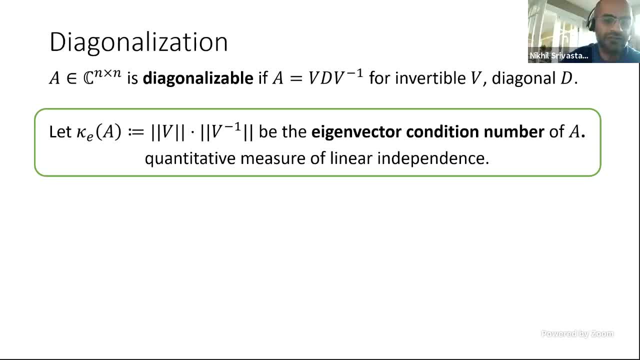 ways to do that, which we'll see in the talk, but one natural one is to look at the eigenvector condition number. So let kappa E of A be the condition number of the eigenvector matrix of A. So you notice that. okay, so the eigenvectors don't come with a canonical scaling, So let's. 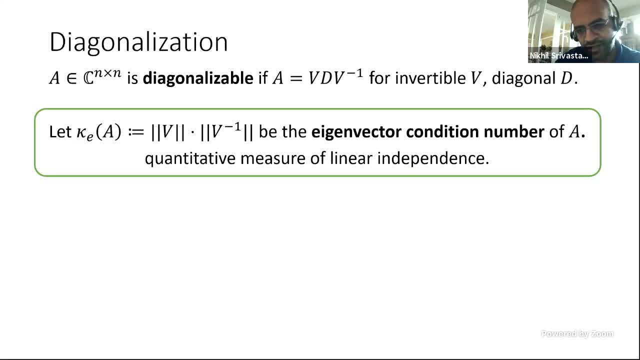 take this to be the minimum of the condition number over all scalings of the eigenvectors. Okay, so that's the eigenvector condition number of A And that's a quantitative measure of how linearly independent the eigenvectors are. So in our three examples here, 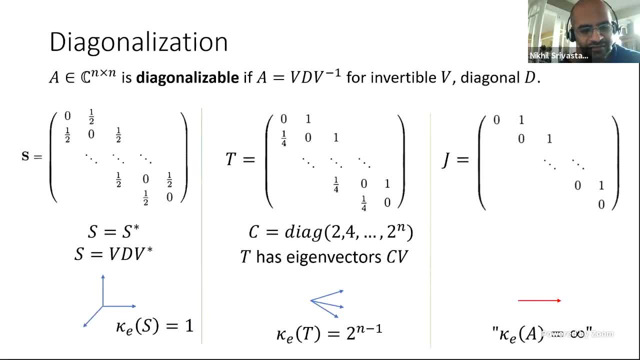 we can calculate this parameter. So in the first example the eigenvector condition number is one, because the eigenvectors are. you know, the eigenvector matrixes are orthogonal. In the second example the eigenvector condition number is actually two to the n minus one. 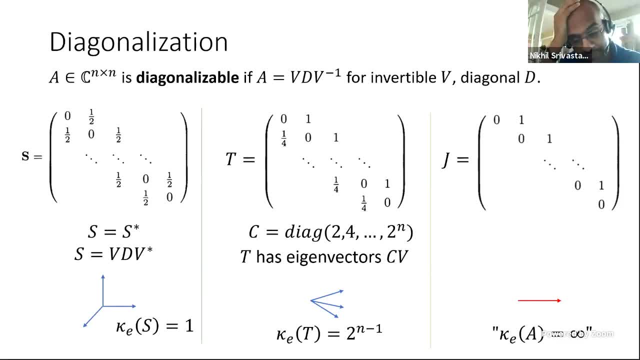 It's just the condition number of the C that we hit the eigenvectors with. Okay, so that reflects the fact that somehow this is less diagonalizable. And then, okay, in the case of the Jordan block, you don't even have a basis of eigenvectors, so you can think of that as saying that the eigenvector 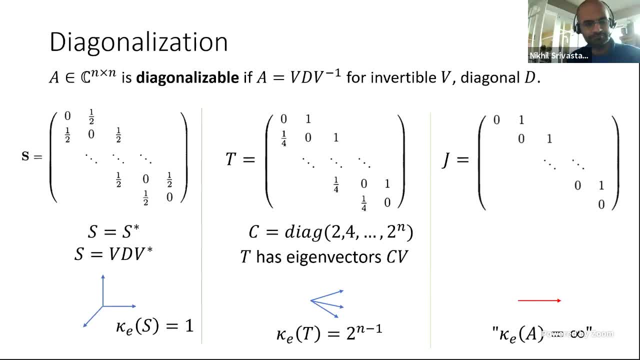 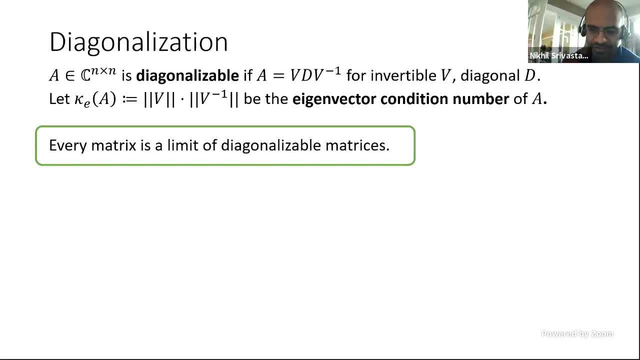 condition number is infinity, So all the eigenvectors collapse into one vector. So okay, so what else do we know? Well, every matrix is a limit of diagonalizable matrices. So diagonalizable matrices are dense. But the question I want to study is this quantitative question. 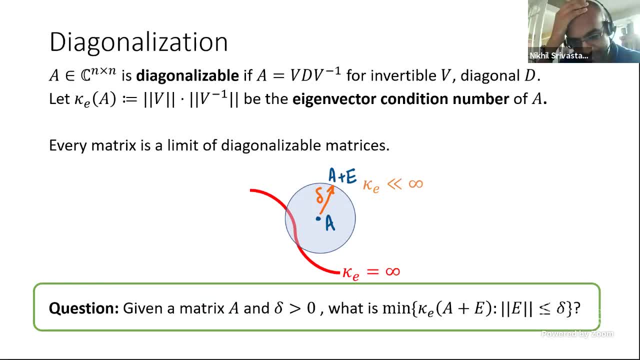 which is given a particular matrix, can you find a nearby matrix that is well diagonalizable? Okay, so, specifically, given a matrix and some parameter delta, can I find a perturbation of size delta such that the perturbed matrix has a small eigenvector condition number? So that's what I mean by well diagonalizable. 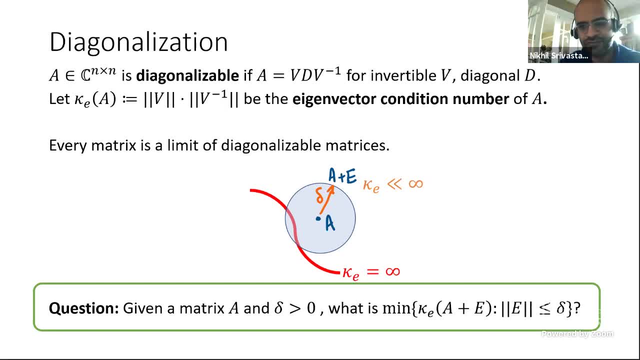 Okay- and this is a quantitative version of this fact- that you can approximate any matrix by a sequence of diagonalizable matrices. Now I'm asking how diagonalizable Okay? so this picture here is sort of a cartoon. This red curve is some, I guess, manifold of 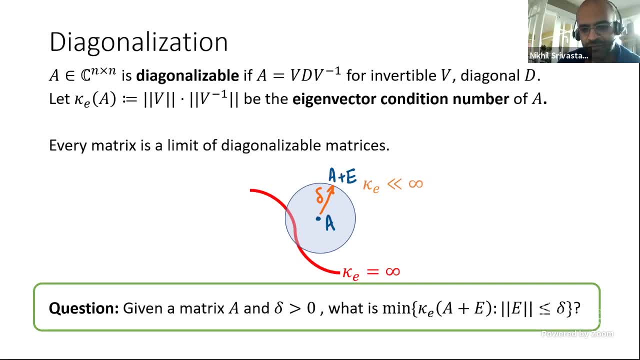 non-diagonalizable matrices and what I'm going to do here after I mean, let me grab that range, and what I'm asking is, suppose I give you some A that may or may not be diagonalizable. I want to find an E so that A plus E has a small eigenvector. 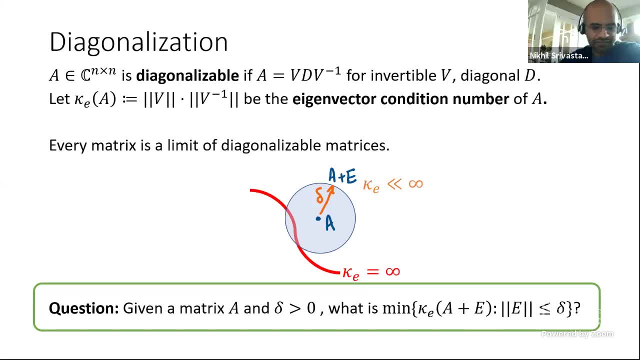 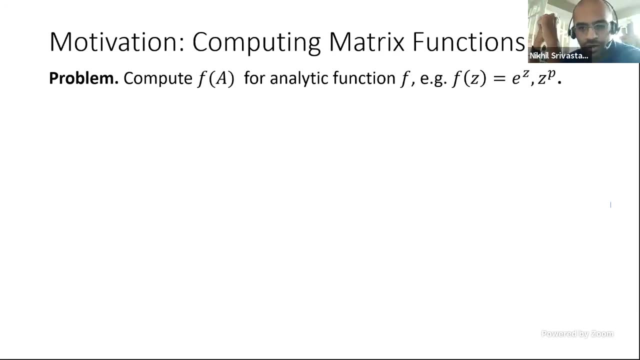 condition number. Okay, so that's a sort of a pretty basic linear algebra question, but the motivation for asking this question actually came from numerical linear algebra, and here's where it came from historically. So here's a problem that comes up in numerical computation. You have a matrix. 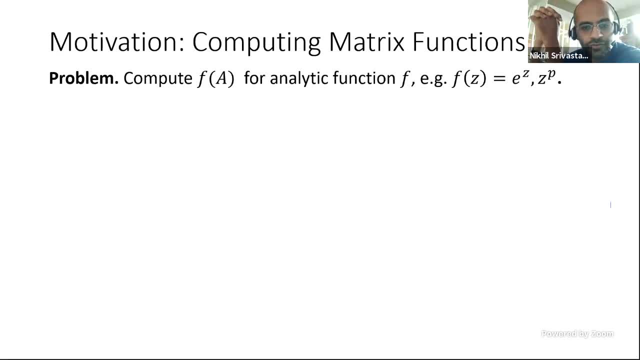 A, which may not be Hermitian, and you want to compute some analytic function, analytic in a neighborhood of the spectrum of that matrix. So, for example, either the Z, that's a nice one, or maybe you want to compute some fractional power. So what does this mean? So what is? what does F of a, even 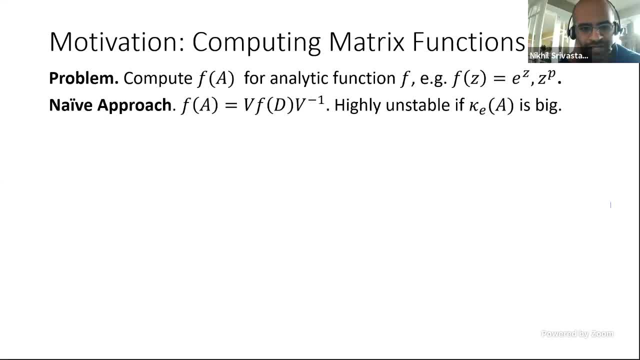 mean? Well, what it means is that if the matrix is diagonalizable, it means that you diagonalize the matrix and apply the function to the spectrum directly. So using this definition, I have that F of A is equal to V times F of B, V inverse if A is. 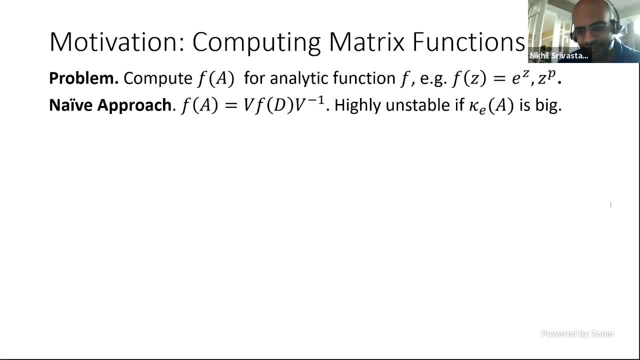 diagonalizable. Well, this gives me some naive algorithm for doing this, but this algorithm is actually not a good algorithm in a lot of cases. So, for example, consider this Toplitz matrix T that I looked at in the first slide. Let's take N equals 100.. So then that's not a. 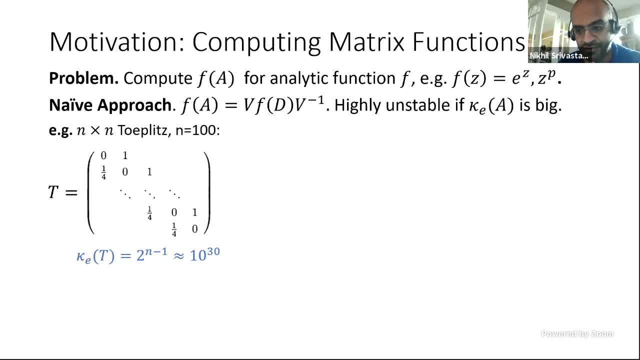 very big matrix. Its eigenvector condition number is 10 to the 30. And so if you try to diagonalize this matrix, you're going to end up trying to invert a matrix whose condition number is 10 to the 30. And you're not going to succeed in doing that. That's way bigger than machine. 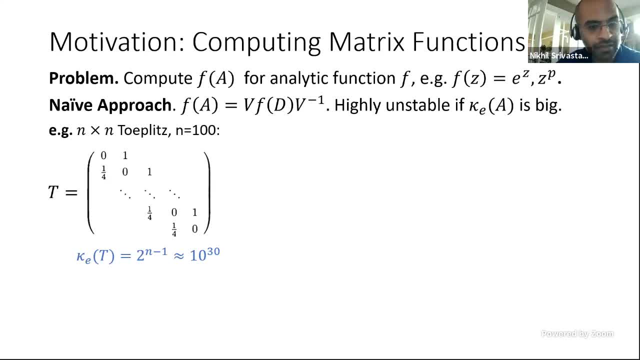 precision, You're going to get some garbage. So what do you do if you want to compute a function of such a matrix? So one empirical observation made by Brian Davies- but this experiment was done by Mark Embry- is the following: 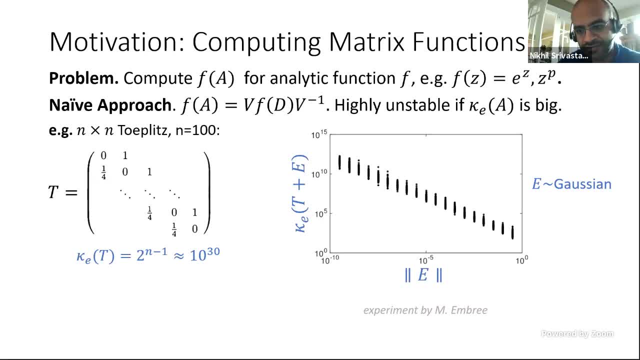 If you take this matrix and now you add a Gaussian perturbation to it, then the eigenvector condition number of the perturbed matrix is much smaller, as indicated in this plot. So on the x-axis you have the norm of the perturbation that you're. 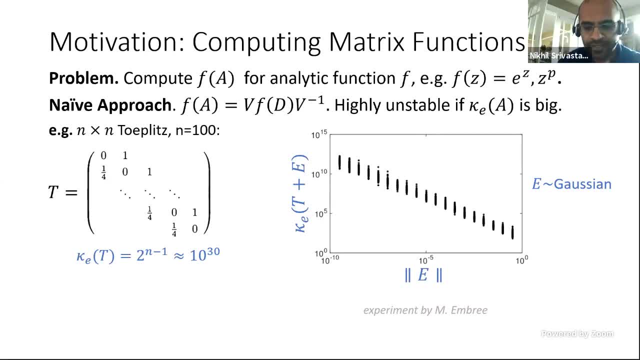 adding, And on the y-axis you have the eigenvector condition number of the perturbed matrix, And what's seen is that you have a Gaussian perturbation to it. And you have a Gaussian perturbation to it. Well, roughly speaking, if you add a perturbation of norm 10 to the minus 5,. 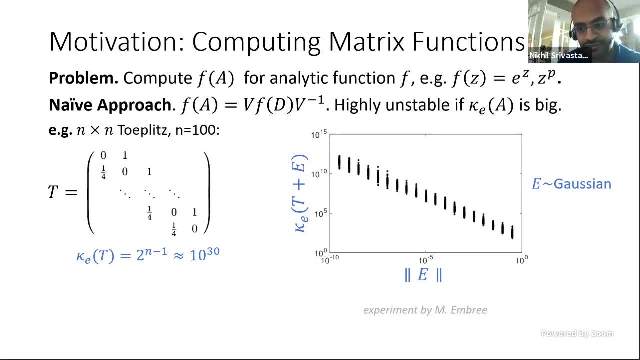 your eigenvector condition number went down to 10, to the 5,, which is very manageable And roughly speaking it appears to be some kind of a linear relationship. So the empirical phenomenon here is that, well, this matrix has a terrible eigenvector condition. 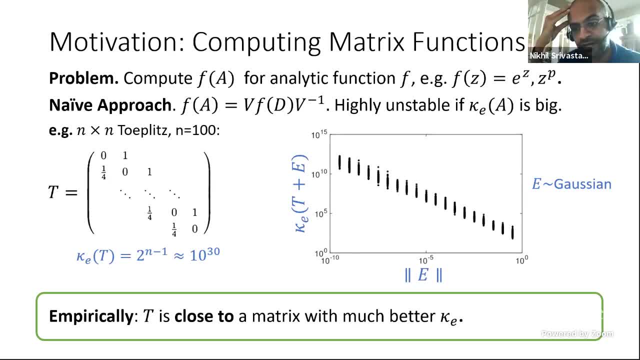 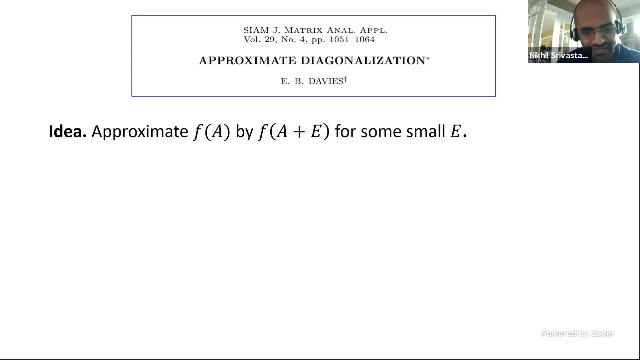 number. but it's very close to a matrix with much better eigenvector condition number. So this led Davies to. So this led Davies to propose the following scheme for computing a matrix: a function of a, not of a matrix. The idea is well, don't compute F of A, Compute F of A, A plus E for some tiny E. 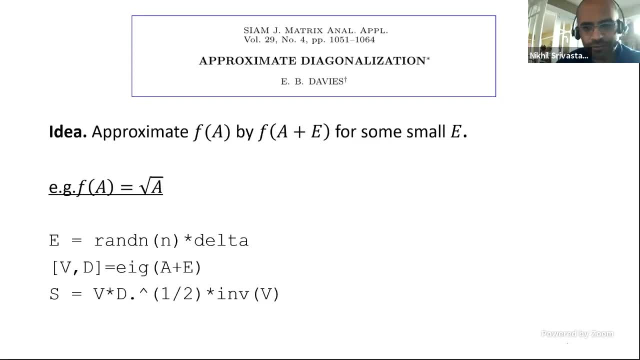 Okay. So, for example, let's say you want to compute the square root of a matrix. So here's a MATLAB code that's proposed in this paper. Well, don't just compute the square root of A First generate a random matrix. So let's say you want to compute the square root of a matrix. 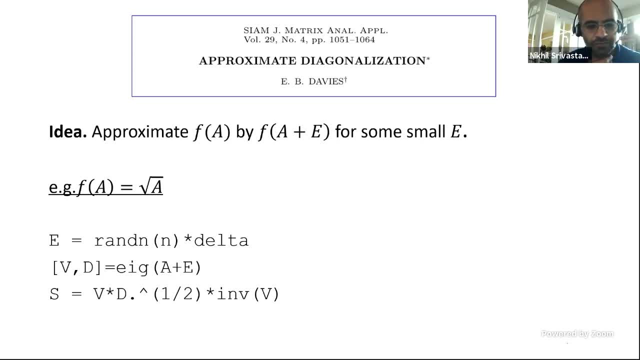 So first generate a random Gaussian matrix times some small delta, Then diagonalize the perturbed matrix and output the naive square root of that matrix. Okay, So diagonalize the perturbed matrix. If that has a small eigenvector condition number, then maybe you should be able to do that. 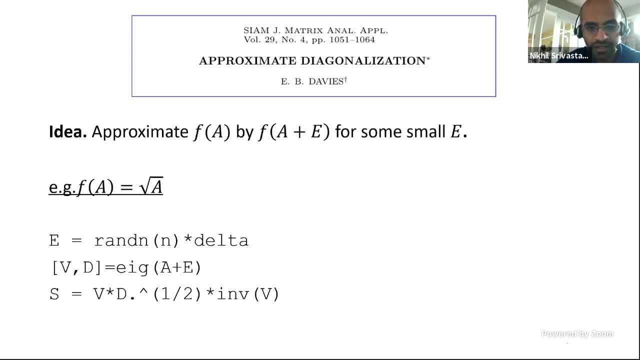 And then output this S. And the nice thing is that this code actually does better than MATLAB square root command on various non-Hermitian matrices. So these are some examples. So let's experiments carried out by Embry where, if you naively just run MATLAB square root, you 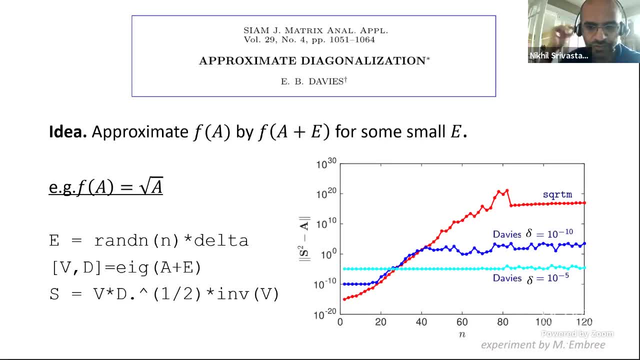 start getting garbage after matrices of size maybe 40. But if you apply this regularizing perturbation before and then compute the square root of that, well, the nice thing is that what you get actually turns out to be much closer to the square root of the original. 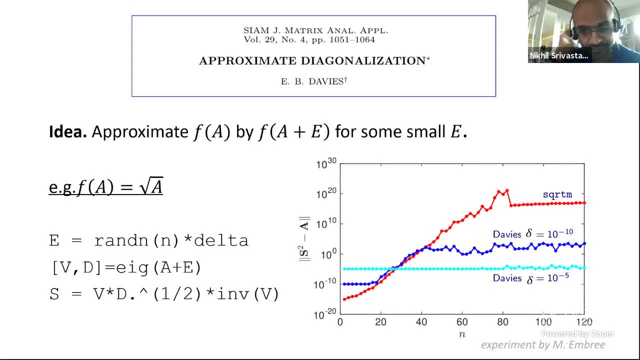 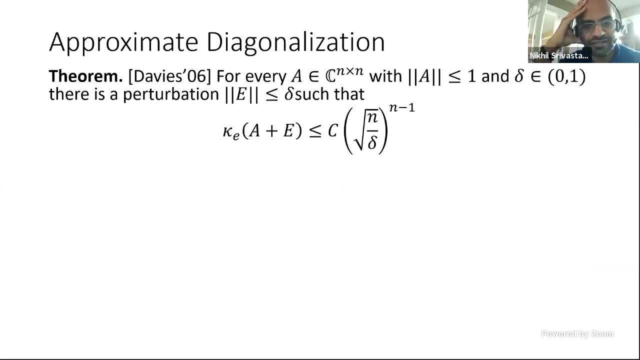 matrix. So adding this random perturbation regularizes the computation. So this led Davies to ask this question that well, what is the dependence of this kappa E on this delta? And he proved the following theorem. So he proved that, given any matrix, 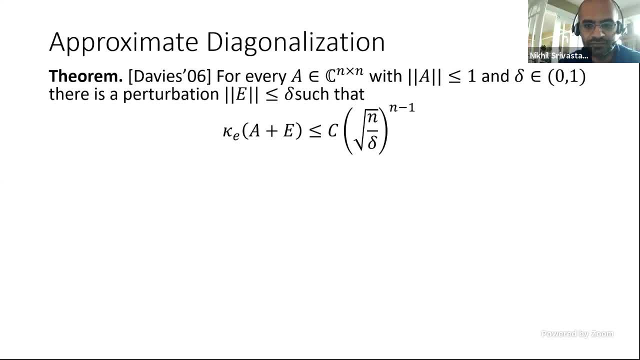 and some parameter delta, there's a perturbation of norm delta. OK, the original matrix has norm 1, so there's a perturbation of norm at most delta. So that when you add this, when you perturb A by this E, this perturbation, E, then the new eigenvector. can turn out to be the same as the perturbation of norm delta. So that when you add this, when you perturb A by this E, this perturbation E, then the new eigenvector can turn out to be the same as the perturbation of norm delta. So that when you add this, when you add this, 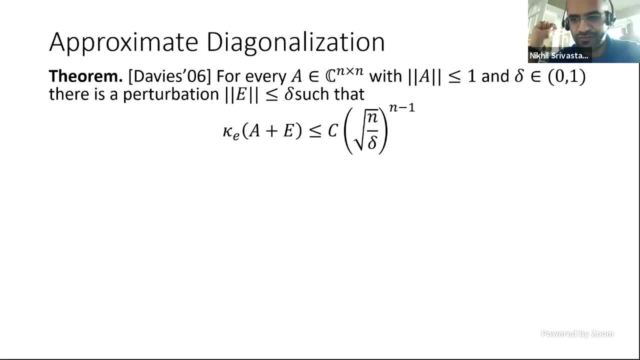 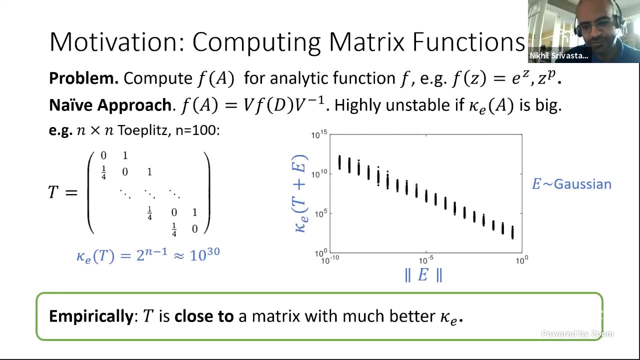 condition number is at most roughly 1 over square delta to the n. OK, so that's what he was able to prove. Now, that's not quite predicting what we saw in the experiment, right? So in the experiment it looked like the eigenvector condition number was decaying. 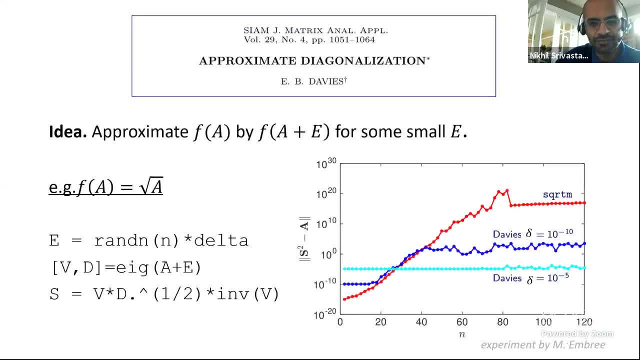 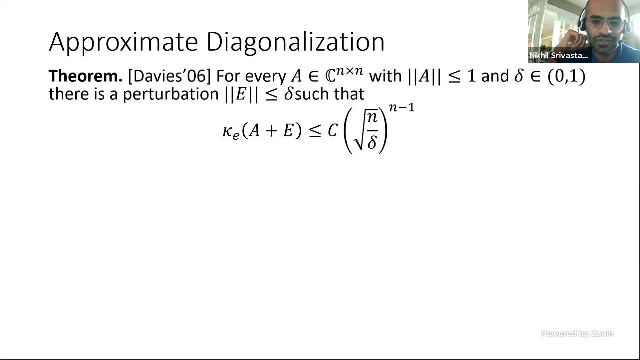 somewhat linearly in the size of the perturbation, whereas this theorem says that. all this theorem proves is that it's at most exponential in 1 over the size. So in particular this theorem is actually not that useful for computation. because you said delta would be, let's say, 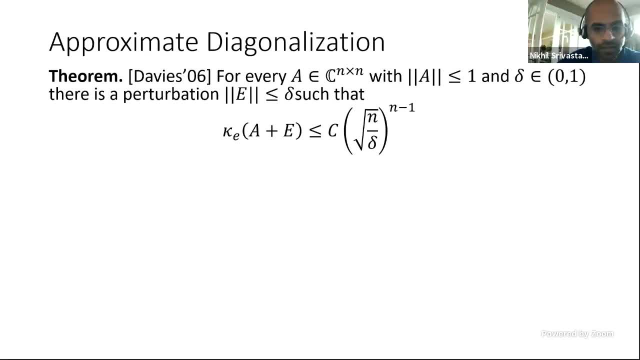 a half, You still get 2 to the n out of this. But Davies made this conjecture that really the right dependence should be inverse linear. So for every matrix A the conjecture is that for every matrix A there exists a perturbation E, so that the eigenvector condition number of the perturbed- 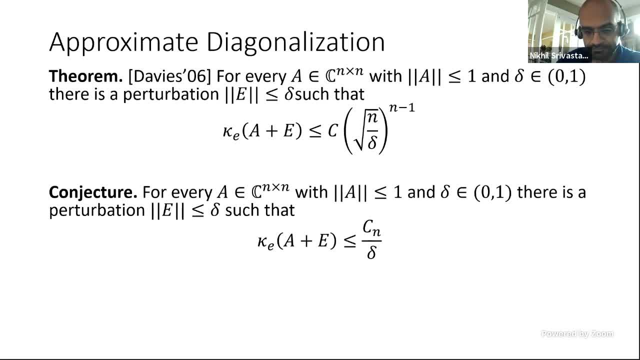 matrix is some function of n over delta And this would be useful in the application I just mentioned. And he proved the conjecture for n equals 3, because the theorem above for n equals 3 actually gives this And he proved it in the special case of A equal to a Jordan block, but didn't prove the 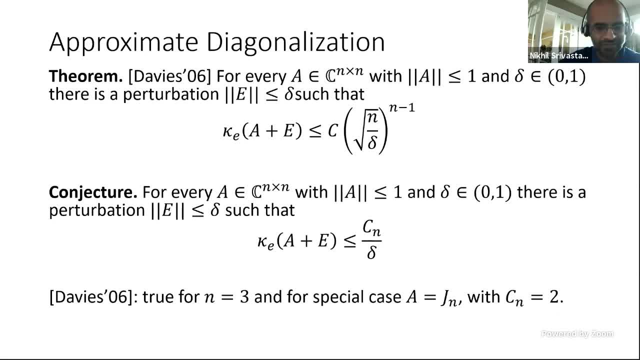 theorem in general. So any questions about the conjecture. I mean, is the conjecture that it exists or is the conjecture that it's high probability? The conjecture is that it exists. Any other In the conjecture I guess there is no probability, right? 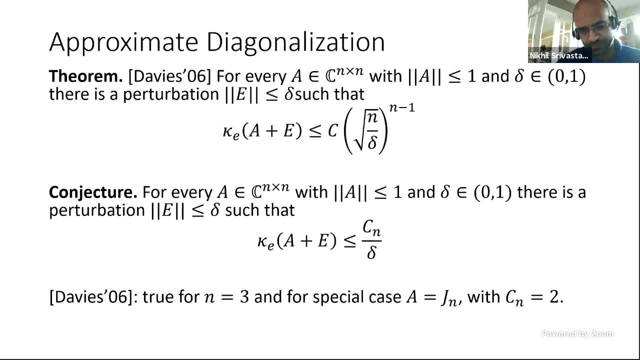 There's no probability. So I'm going to solve the conjecture by proving that it with probability, but the original conjecture is just about existence. Okay, So the first theorem I want to talk about is that the conjecture is true. So the theorem is. 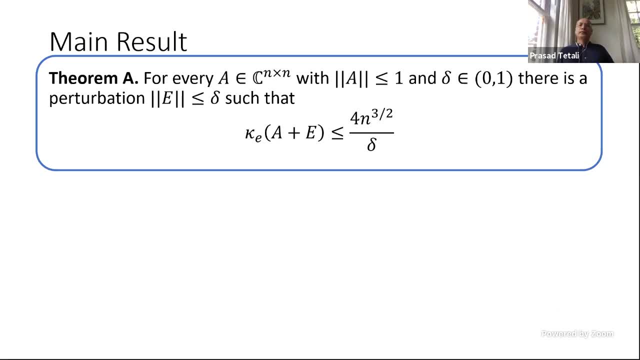 that. yes, this is true, and the dependence is 4: n to the 3 halves over delta right Every A, there exists a perturbation E of norm delta, so that this is true. So in particular, it means if you set the perturbation to be 1 over poly n. 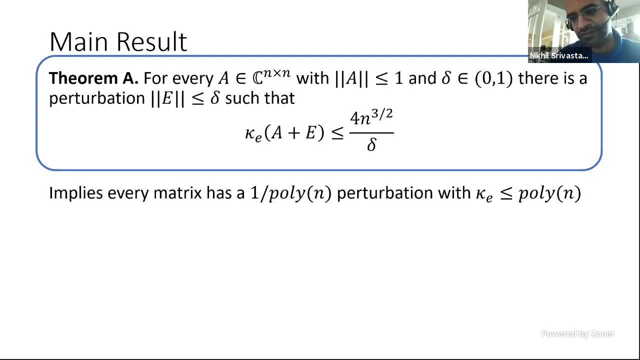 it means every matrix has a 1 over poly n size perturbation with eigenvector condition number poly n And, as anticipated by many people- this is, you know, such as Galena's question right now- this is implied by a probabilistic result. But the probabilistic result is actually about 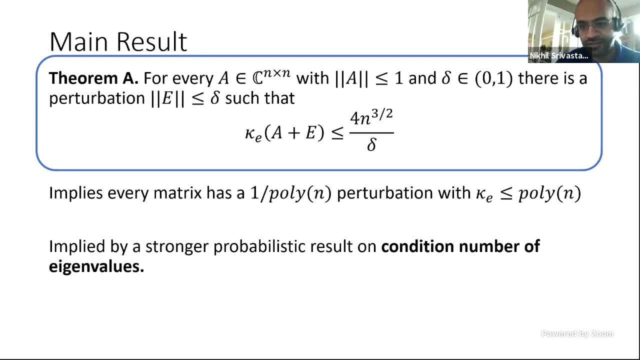 you know a different related quality called the eigenvalue condition number. Okay, So any questions about the statement of the theorem. before I move to that, I guess, do you expect it to be tight? You mean this bound? So we proved that the dependence on delta is tight. 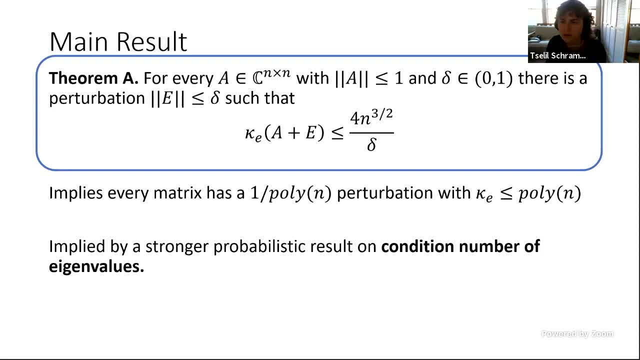 We don't know about the dependence on n. Thanks, Do you know if there should be a dependence on n? No, So in fact there's a 1989 conjecture From operator theory that there should be no dependence on n. 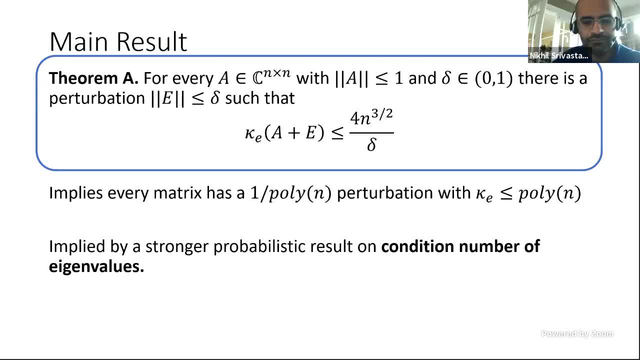 possibly at the cost of some other dependence on delta. yeah, I'll mention that at the end. May I ask if you could remind what is the dependence that Jain and Sinval got in the real version? Was it different That who? excuse me? 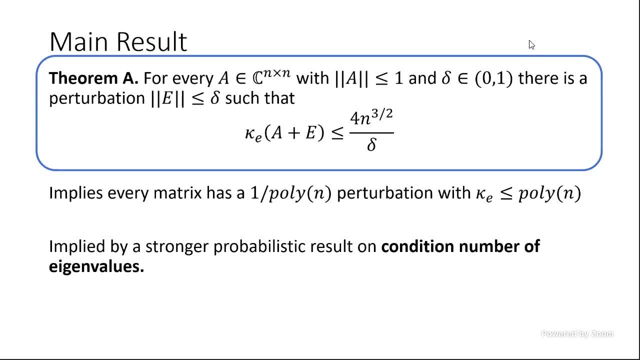 Well, Jain and Sinval, I might be. Ah, yeah, I'll talk about that later. Yeah, yeah, yeah, So that's a sort of follow-up of this result. I'll talk about it later. Okay, So that's a sort of follow-up of this result. I'll talk about it later. 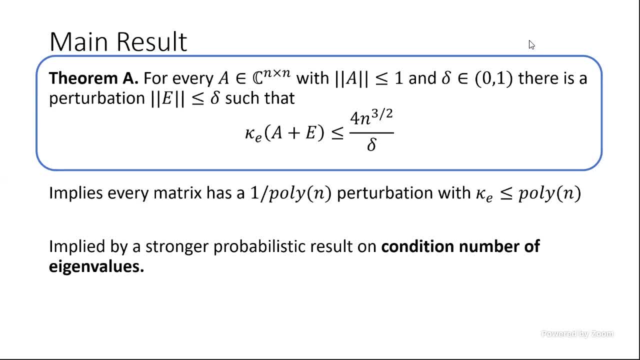 Okay, So that's a sort of follow-up of this result. I'll talk about it later. Mm-hmm, Okay, They got almost the same thing with the log delta, I see. Okay, So what is a condition? number of eigenvalues. 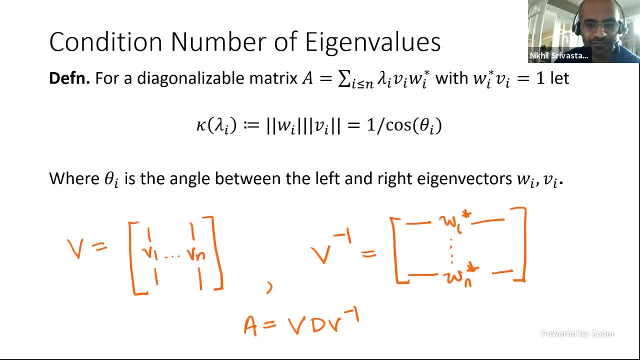 So let me define it. So suppose you have a diagonalizable matrix A with distinct eigenvalues. I'm only going to define it for distinct eigenvalues, And now I'm going to write its spectral decomposition additively as summation. lambda i vi wi star. 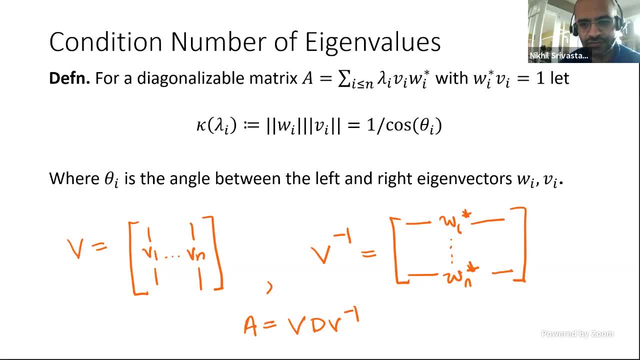 So wi star. So the left eigenvectors, vi are the right eigenvectors. They're normalized to have wi star, vi equals one. So if you look at these matrices, v and v inverse, the wi star are the rows of v inverse. 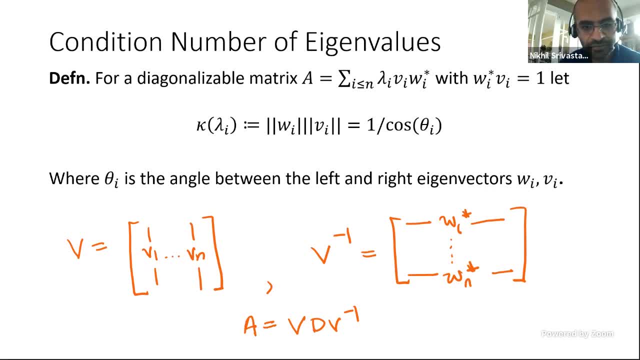 So the eigenvalue condition number of the eigenvalue lambda i is the norm of wi times, the norm of vi. Okay, So these are vectors that are not unit vectors. They're normalized to have inner product equal to one. That's what it means to have v times v inverse equal to one. 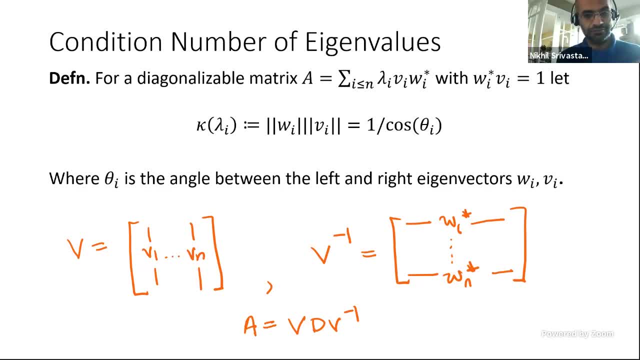 But for non-Hermitian matrix you know their norms could be way, way bigger when you make this normalization. So this eigenvalue condition number is one over the cosine of the angle between the left and right eigenvectors. So in the Hermitian case these numbers are all equal to one. 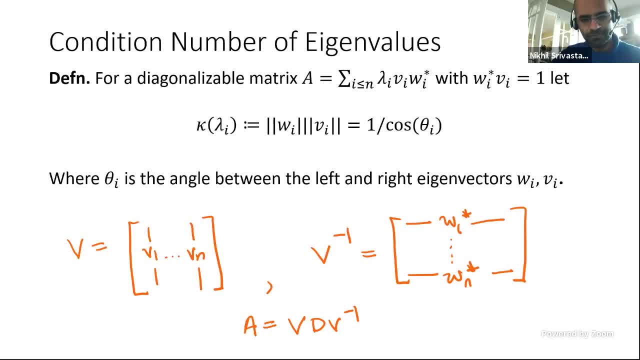 because the left and right eigenvectors are the same. But as you become more and more degenerate, this blows up. So why is this called the eigenvalue condition number? So it turns out, this is the number that controls the speed of perturbation of any particular eigenvalue when you add a tiny perturbation. 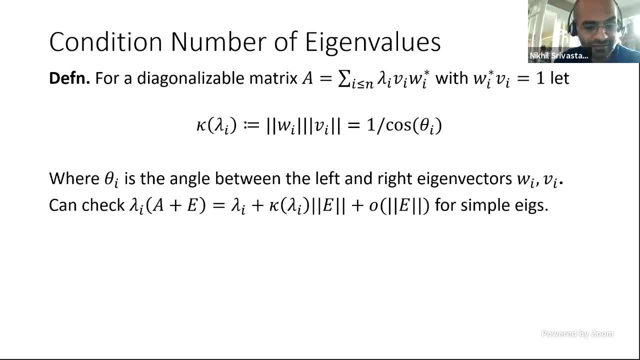 So if you look at a plus e and you look at lambda i, some eigenvalue. well, this is saying that if you apply a tiny perturbation, then the perturb eigenvalue is the size of the perturbation times. this eigenvalue condition number. 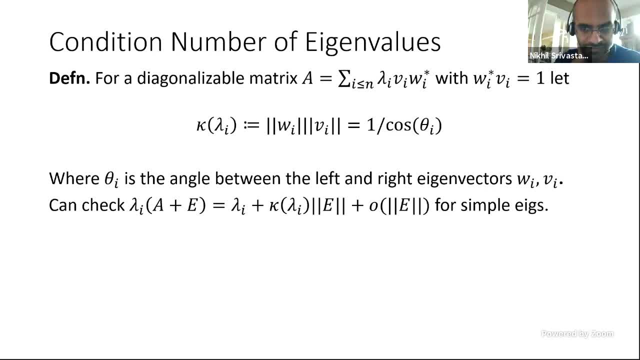 So this measures the sensitivity of a particular eigenvalue to perturbations. Okay, And this is all well-defined because eigenvalues are simple. So this is now another measure of quantitative diagonalizability, right? So small eigenvalue condition numbers means somehow strongly diagonalizable. 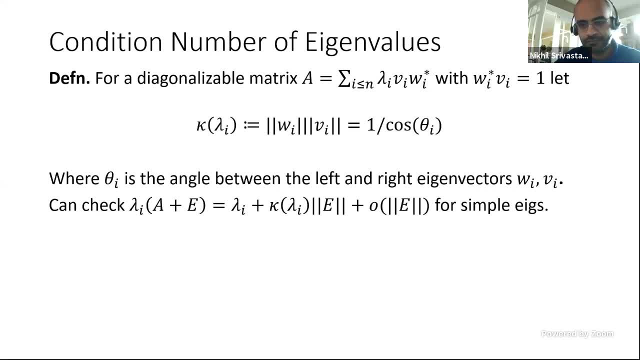 That's what I'm going to take it to mean, But in particular it means that the spectrum is stable. You can actually be. the norm of e appears in the filter, So can you get the perturbation, which is it does not affect lambda at all. 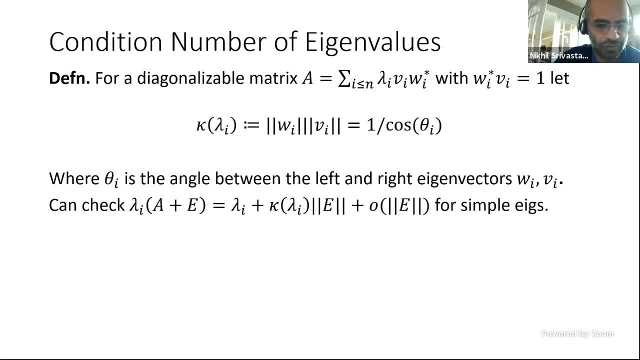 How come you always get: Oh, I'm sorry, I'm sorry, So what's written here is It's sort of, in the worst case, Oh, okay, Yeah, sorry, So what's written here? You're right, You can find a perturbation that doesn't affect lambda at all. 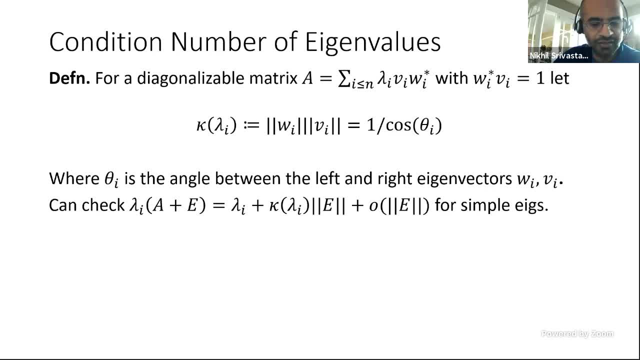 Just move along some other eigendirection. So you're right. I should say that the size of the perturbation is upper bounded by this quantity. So would the direction of this bad perturbation, I guess, be b i w i star. 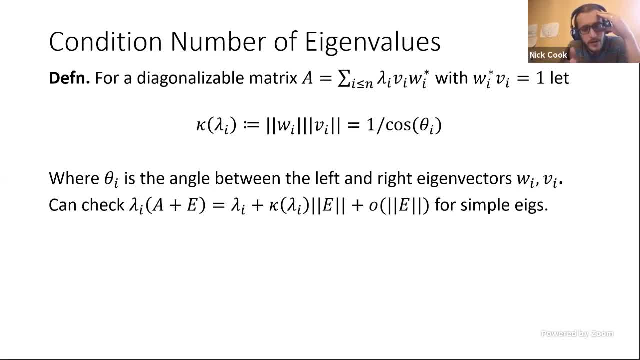 The direction of this bad perturbation. Yeah, So there's a worst case, So there's a worst case direction which would be in that rank one. Well, actually, no, No, no, no. So if you take e equal to v, i, w, i star, then I mean, normalized this way the norm of e. 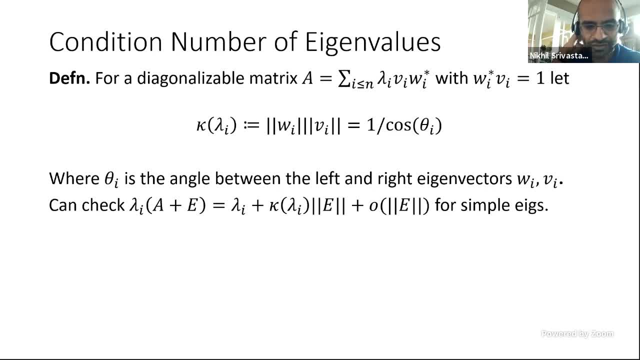 itself is already very big. So actually the bad direction is not actually v? i w i star. If you add a spectral projection, It's not a, Is it not just a? Yeah, If you take e, Wouldn't you just scale the eigenvalue? 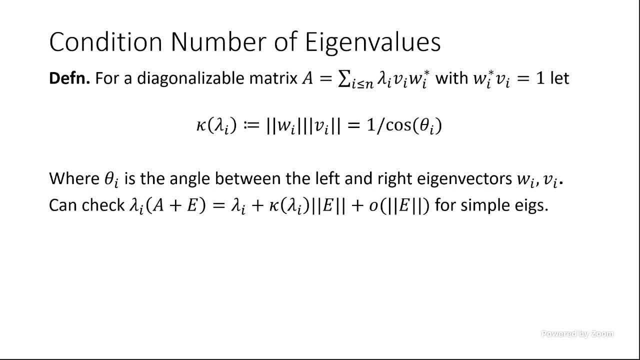 Okay. So if you just move by a, Okay. So I'm thinking of this kappa lambda i as being a very big number. So if you just add a multiple of a, then the eigenvalue is just going to. If you look at a plus delta a, let's say right. 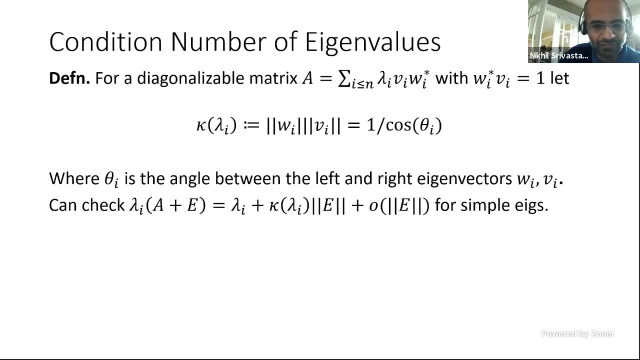 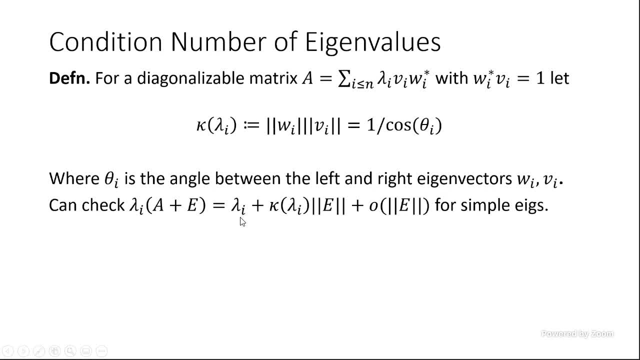 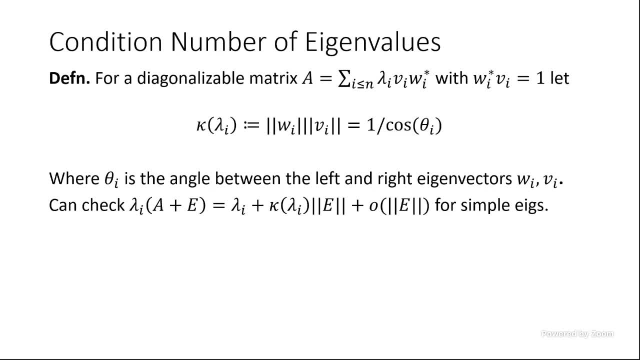 Well, the eigenvalues are complex so I'm not necessarily assuming they're ordered Okay in any way, The Okay fine. So if you take the derivative of lambda i, Let me just say, if you take the directional derivative of lambda i and the direction, 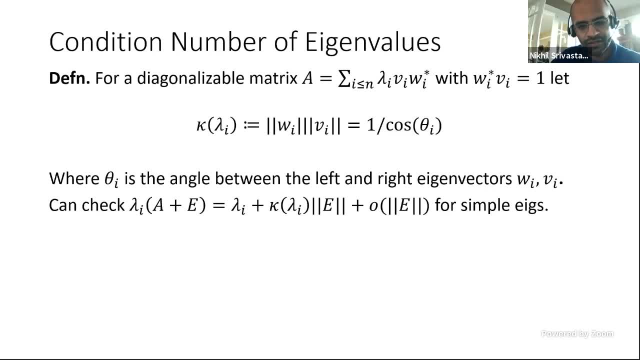 e. it's equal to the quadratic form w star e, v. Okay, And these W star and V. so the point of this is what this is saying is that if W, star and V have big norm, then this perturbation is large. 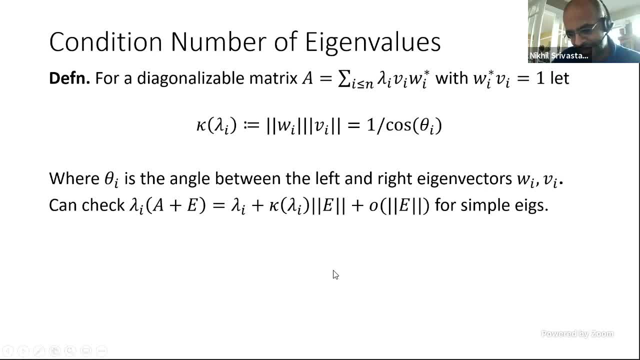 Oh, I'm sorry. Okay, now I see what Nick is saying. You're right. So if you want to maximize that over, let's say, matrices of unit, norm you- yeah, I guess you would take W V star. 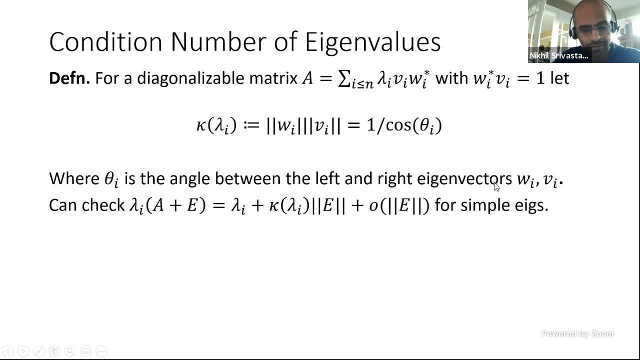 Okay, thanks, Yeah, sorry to No. no, no, sorry, I misunderstood the question. Yeah, Okay, so so this is related to the eigenvector condition number in the following way. It's: it's polynomially controlled on both sides by the the eigenvalue eigenvector condition number is polynomially controlled by the largest eigenvalue. 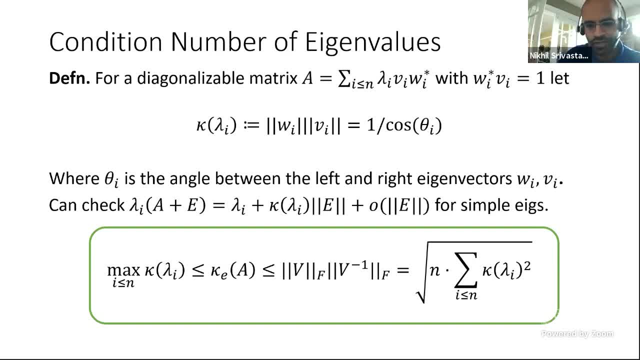 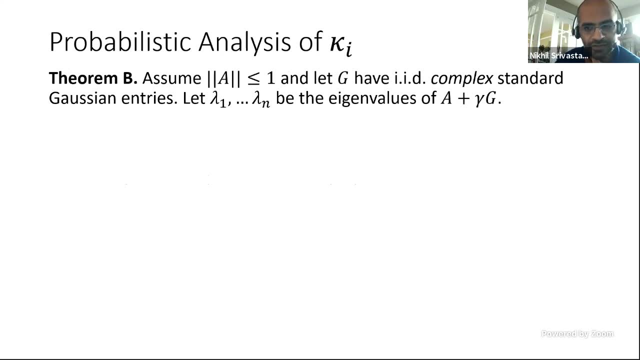 So it's the eigenvalue, condition number and some, you know, root n times the sum of its squares. So up to polynomial factors, these quantities are relatable, for any matrix is a deterministic statement, Okay, So now? so let me mention now theorem B, which implies theorem A. This is a probabilistic theorem. So suppose A is a matrix of bounded norm. and let's take G to have IID, complex standard Gaussian entries. 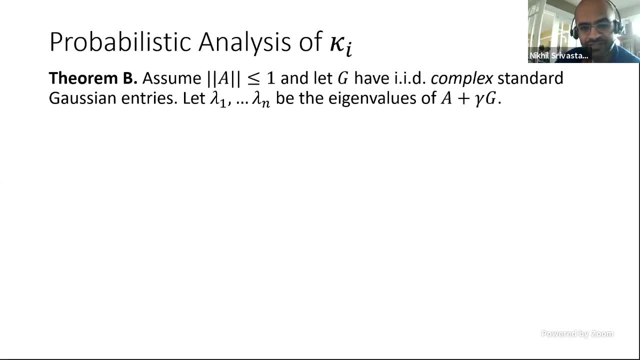 Then with probability 1.0.. The eigenvalues of A plus Gamma G are distinct. So Gamma some positive parameter And call these eigenvalues lambda one through lambda n. And if you a complex standard Gaussian means it's a Gaussian in the complex plane where the real and imaginary parts have variance one half. 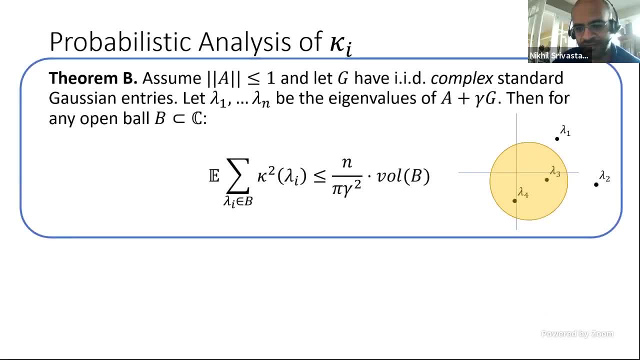 So okay, then the theorem says, if you fix any open ball B in the complex plane- So in this picture I fixed this yellow disk And you look, if you look at the average of the sum of squares of the eigenvalue Condition numbers, of the eigenvalues that land in that disk, that's bounded by n over Gamma squared times the area of the disk. 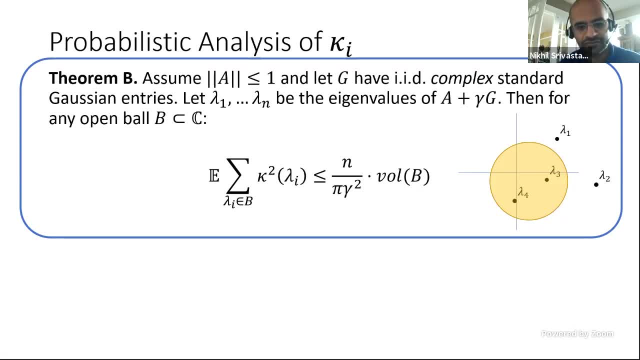 Okay, so the eigenvalues are random, right? So this the sum is over a random subset of the eigenvalues. So you fix B in advance and then over over only the eigenvalues that land and B, the sum of squares of the eigenvalue. condition numbers is bounded as such And the right hand side you can see is: 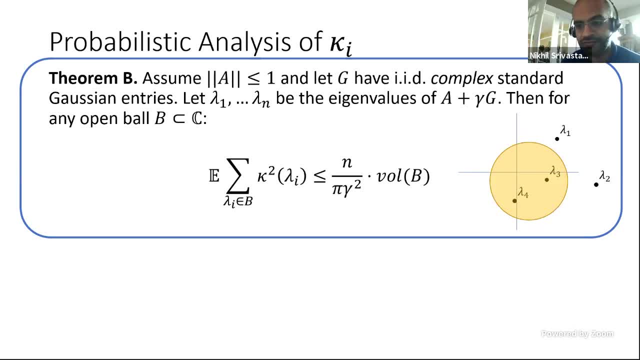 you know, depends in some very nice way On and and on the size of the perturbation. Okay, so This theorem you can. you can compare this to existing theory theorems in the random matrix theory literature. so People have studied in great detail The case of equals zero. So what happens if you just have a pure complex Gaussian matrix? 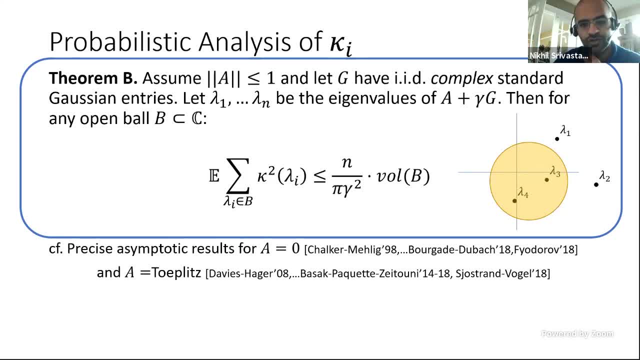 And in that case they're very precise as some products for the joint. you know, limiting distribution of these eigenvalue condition numbers- You're starting with Chalker and Milligan, most recently do do or God do back and Fedora, And also in the mathematical physics literature people have studied in great detail The case when a is a topless matrix. 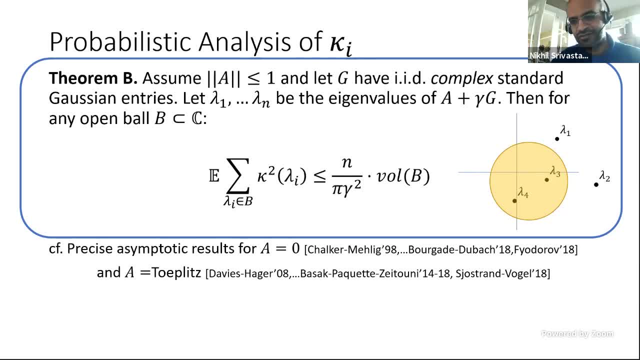 And again they've proved some various precise limit laws for the distribution of these eigenvalue condition numbers. In contrast, what we prove is Much coarser. It's just an upper bound on the expectation, But it's true for any a and it's totally non asymptotic. 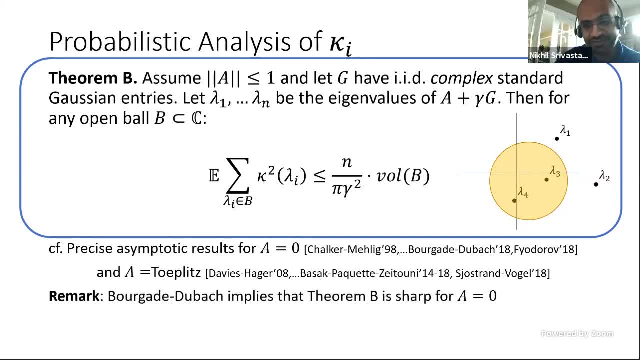 And I should mention that some of these random matrix here results imply that this theorem is sharp in its dependence on n and its dependence on gamma. It's actually sharp in the case a equals zero. So any questions about the statement of theorem B, So n in particular cannot be replaced by say how many lambdas land inside B. 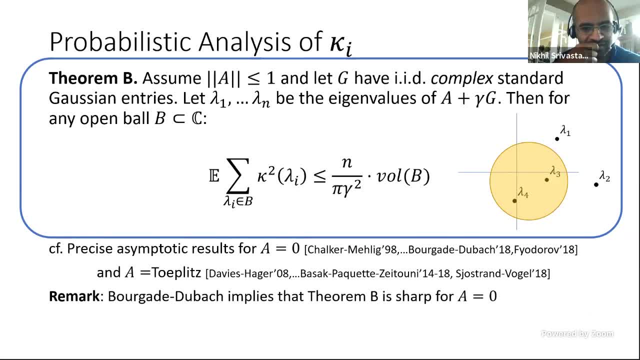 Okay, so I should be precise about the quantifier. So it's sharp in the sense that if you fix for there's a particular B for which the dependence on n is sharp. I don't know if you can replace n by the number of eigenvalues. 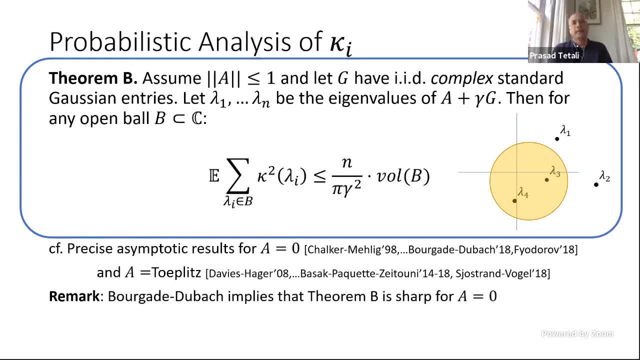 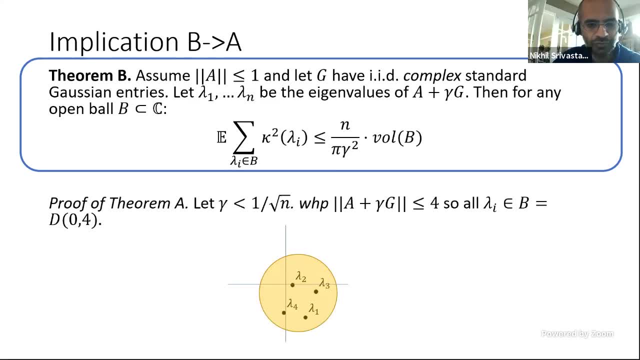 Okay, so how does this imply theorem A? Well, it implies theorem A in a pretty straightforward way. So what? What's the proof of theorem A? I'm given a matrix A. I need to find this perturbation E. I'm going to take E to be gamma times G, where G is a complex Gaussian matrix. 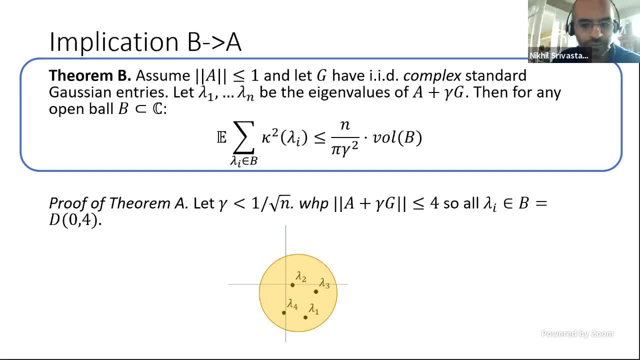 And let's assume gamma is less than one over square root n. That's the right normalization, because the norm of G is two square root n with high, at most two square root n with high probability plus little over one. So then some standard random matrix here results tell us that the norm of A plus gamma G is less than four with very high probability. 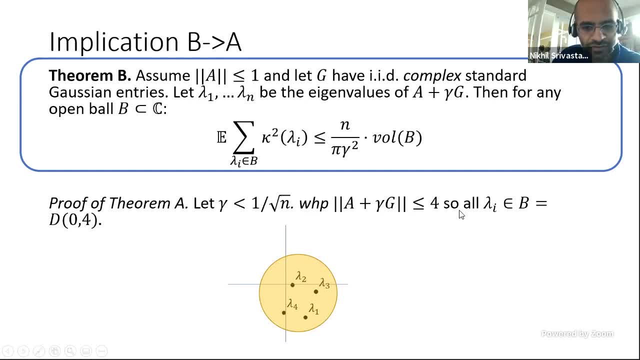 Okay, A is normalized to have norm less than one. So then, with very high probability, actually all the eigenvalues will lie in a disk of radius four. So what I'm going to do is I'm going to invoke theorem B with a disk of radius four in the complex plane. 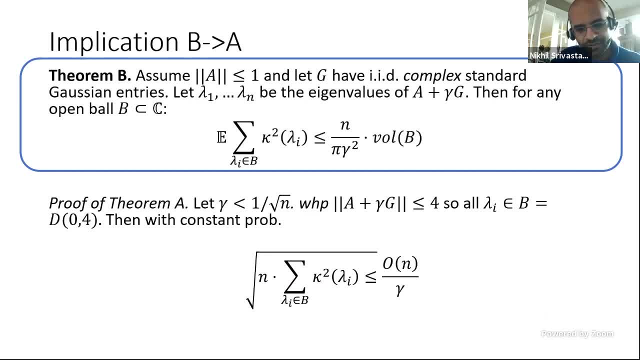 So what does theorem B say? Well, just by Markov, it says that, with constant probability, the sum of squares of the eigenvalue condition numbers of the eigenvalues in that disk are bounded by n over gamma squared times the area, which is some constant. 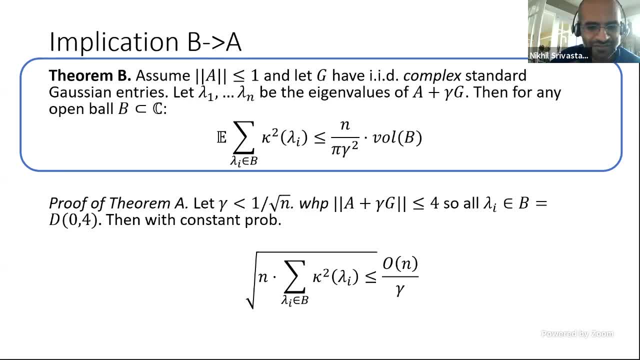 So now if I take that and multiply by n and take the square root, that says that that quantity is bounded by n over gamma, right, So I have n times n over gamma squared. the square root of the whole thing is n over gamma. 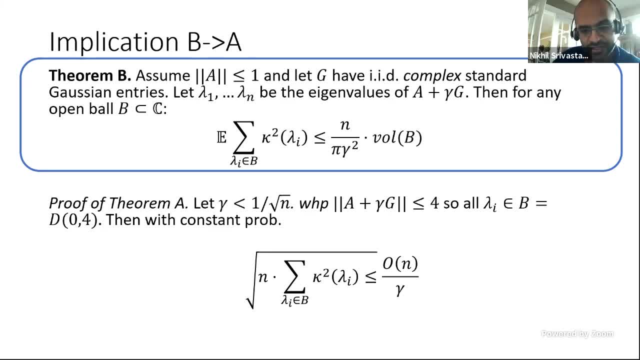 So now I take a union bound so I have a constant probability this holds. But, as I said, all the eigenvalues land in the disk. So the sum of our eigenvalues in B is the sum of all eigenvalues. And you know I showed you earlier that this is an upper bound. on the eigenvector condition number: 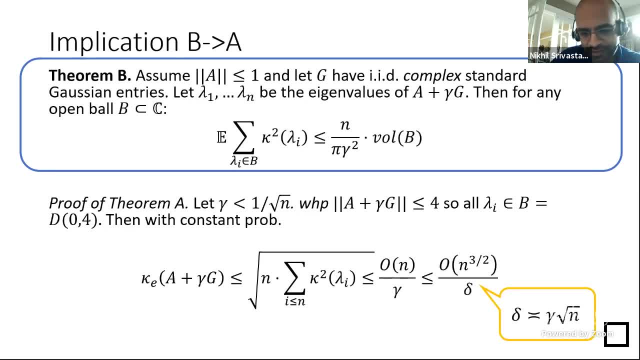 So. so then that's it right, Because now the size of the perturbation is gamma times, the norm of G, which is gamma times squared n, And so, in terms of the size of the perturbation, the eigenvector condition number I get is n to the three halves over delta, which was what was advertised. 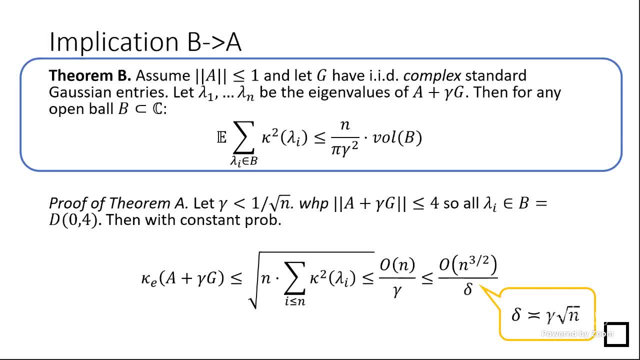 Okay, Can I ask a question? Yep, So for theorem B the upper bound does not depend on the location of the ball right, But if the ball is very, Very far away from origin, you would expect the number of eigenvalues smaller there. 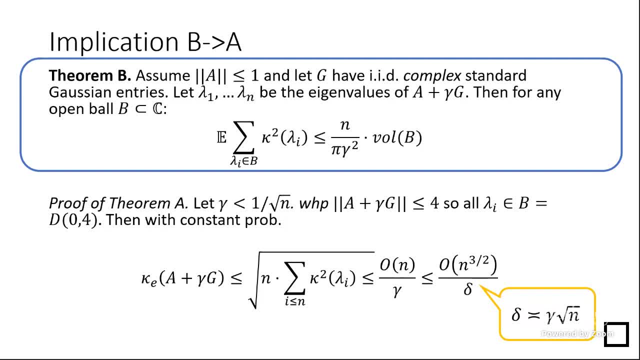 So is there like yeah, is there some intuition about bound or why is it looking like this? Well, so I mean okay. So one intuition related to the theorem is that unstable eigenvalues will tend to move randomly. Okay, So let's say, I choose a tiny ball around an eigenvalue, right? 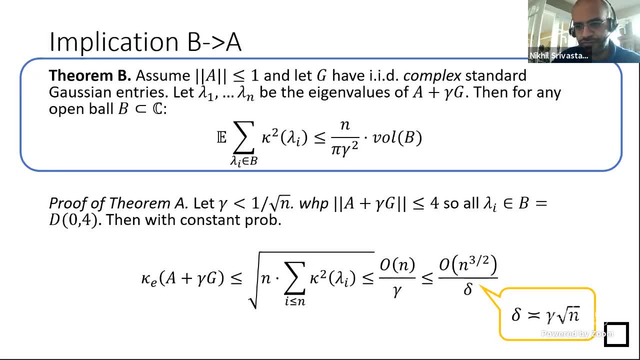 So you know, let's say I have fixed A, I have one eigenvalue and I choose a tiny ball, So then the volume of that B will be very tiny, right, So the right-hand side will be tiny If that eigenvalue is unstable. what this theorem is saying is that most likely it's going to leave the ball. 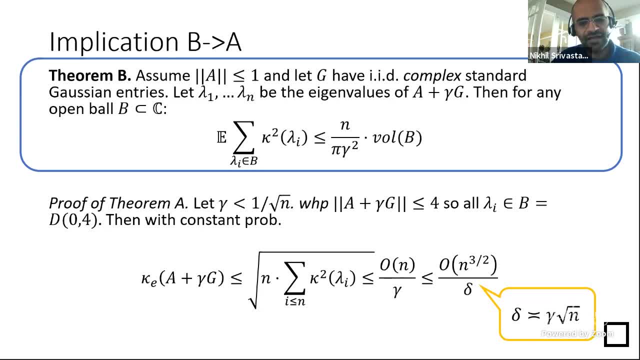 Does that make sense? So unstable eigenvalues cannot be concentrated in a small region of the complex plane. That's what the theorem is saying. after applying the random perturbation. Okay, But you're right, You have to apply the theorem judiciously. 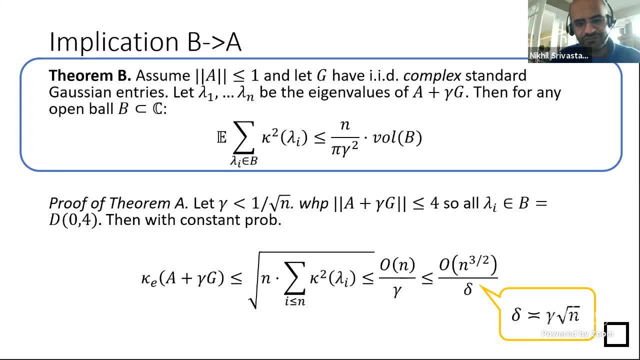 If you choose a ball, that's If you choose a ball that's too far away from the spectrum, the left-hand side should be zero and you'll get some bound on the right-hand side. So you have to choose B somehow judiciously, you know. I mean, if you want to get a meaningful conclusion. 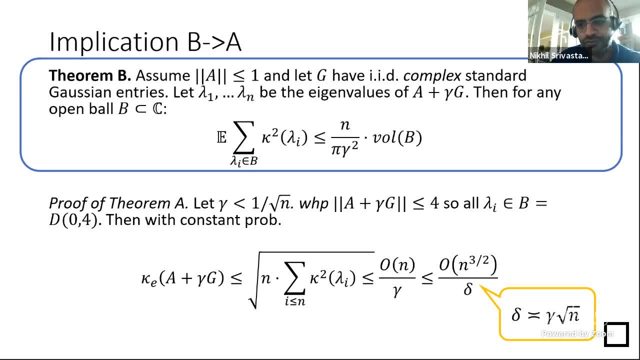 Okay. Is there also a high probability analog of the theorem? No, So this stuff, this distribution, is known to be heavy-tailed, so it actually doesn't even have finite second moment. So there's no high probability analog, Okay. So in particular, that means that this Markov that I did in this little argument cannot really be improved. 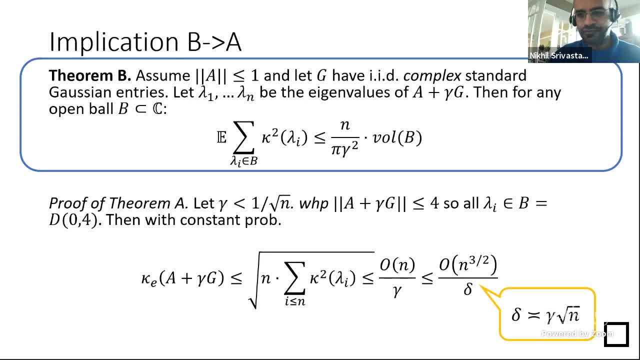 Okay, So now let's prove theorem B. Any more questions about theorem B? So what I've achieved so far is I've gone from the eigenvector condition number, which was somewhat intimidating quantity involving all the eigenvectors, to studying eigenvalues. 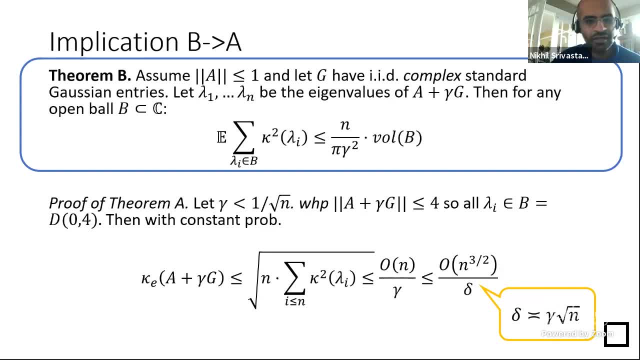 So what I've achieved so far is I've gone from the eigenvector condition number, which was somewhat intimidating quantity involving all the eigenvectors, to studying eigenvalues, To having acker skewed- Miss you- condition numbers, which are somewhat more local quantities, and now I'll show how to analyze that using the notion of pseudo spectrum. 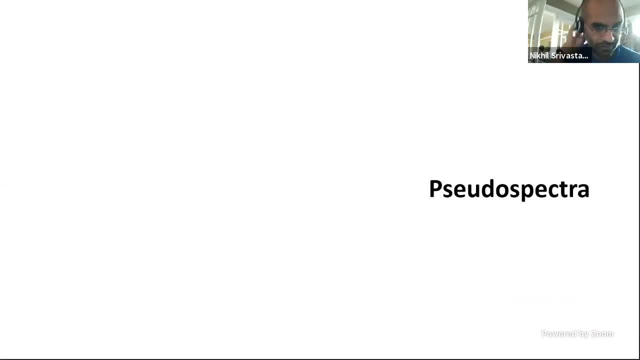 So what I've achieved so far is: I've gone from the eigenvector condition number, which was somewhat intimidating quantity involving all the eigenvectors, And now I'll show how to analyze that using the notion of pseudo spectrum. Okay, so, uh. so what is the pseudo spectrum? 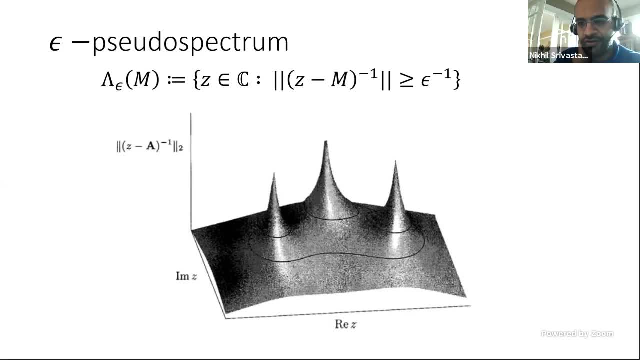 So The pseudo spectrum of a matrix is a set in the complex plane parameterized by a parameter, epsilon. So the epsilon pseudo spectrum of a matrix M is the set of points in the complex plane where the resolvent, which is z minus M inverse, has operated norm bigger than one of Epsilon. 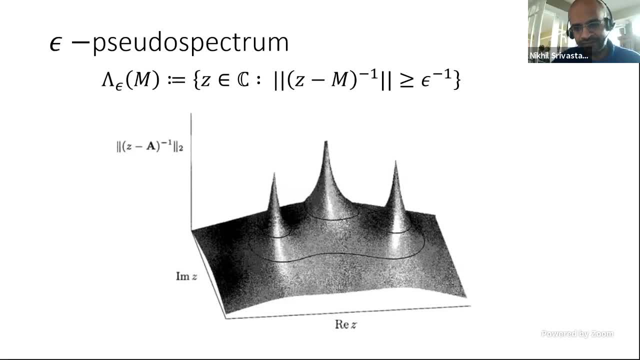 Okay, so this is a picture of some matrix with three eigenvalues And I guess it's a plot of the norm of the resolvent And the peaks. so the poles of this function are the eigenvalues, right? So the resolvent has poles at the eigenvalues. 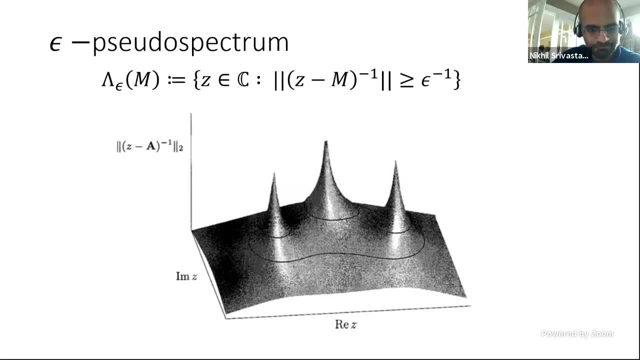 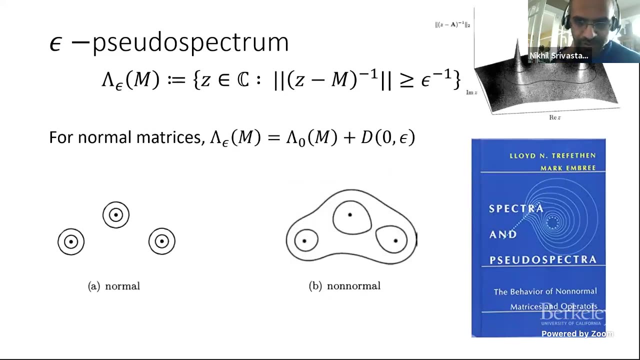 And the pseudo spectrum is asking: well, what are the level sets of that function? So as you make epsilon smaller, these sets become smaller because it's a level set of the resolvent being larger. So there's a beautiful book that I highly recommend about this. 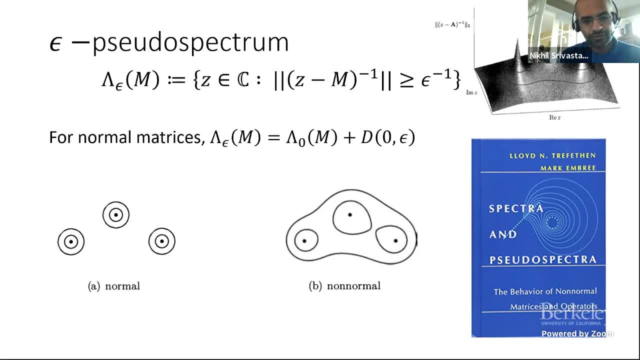 But OK, what do these sets look like? Well, for normal matrices it's very straightforward to see that the pseudo spectra are just disks of radius epsilon around the spectrum. So if M is normal or Hermitian, then the pseudo spectrum is just disks of radius epsilon around. 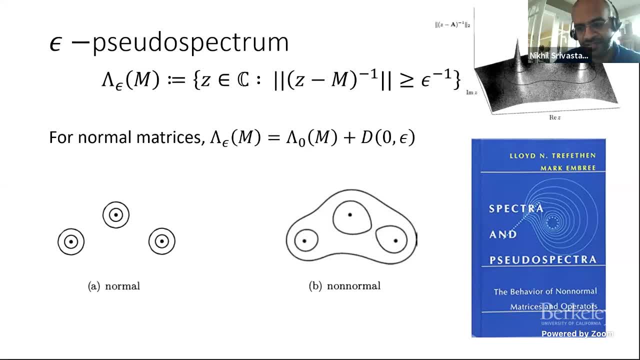 the spectrum, But for non-normal matrices it can look like this. It can look a lot more interesting. So this is a picture of the pseudo spectrum of some non-normal matrix. Now, what does this have to do with diagonalizability and spectral stability? 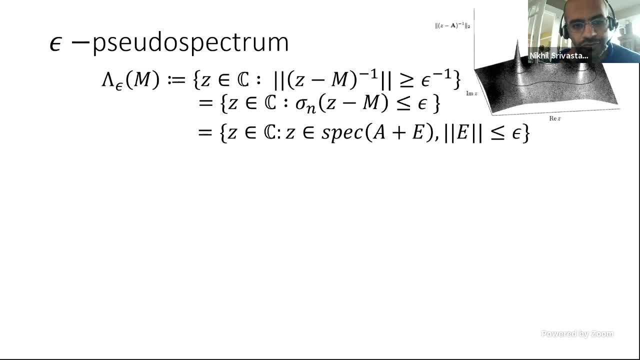 Well, there are these two alternate characterizations of the pseudo spectrum. So this is equal to two other sets. So the first is a set of points z, where the least singular value of z minus n is less than epsilon. This is a triviality. 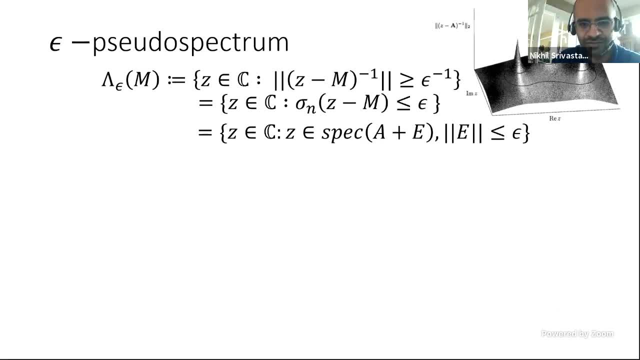 This is just because the norm of z minus m inverse is equal to 1 over the least singular value of z minus n. So it's a set of shifts z, so that the shifted matrix has a small least singular value. And then a slightly less obvious equality is that it's the union of the spectra of all. 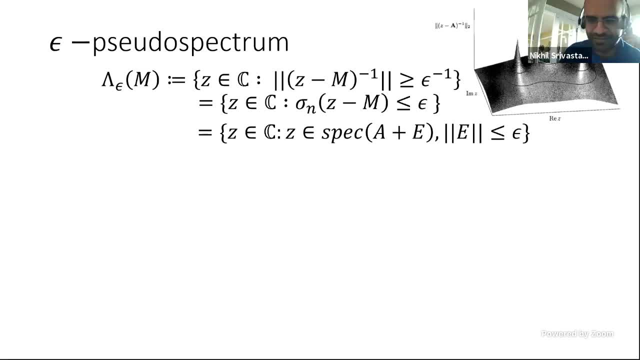 perturbations of A of norm less than epsilon. So this is a very nice exercise which I encourage you to do if you want to get a feel for this, And this is why it's a very relevant quantity for spectral stability. It's the set of all possible eigenvalues you can get by perturbing the matrix M by a matrix. 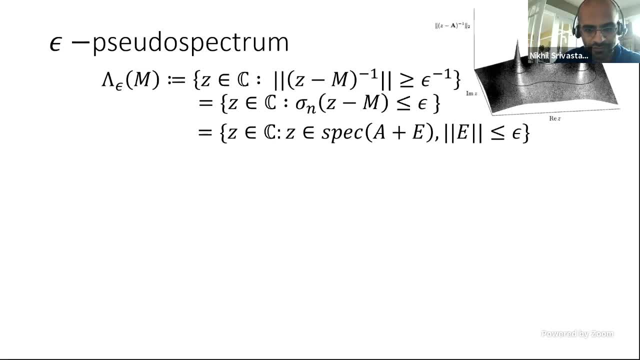 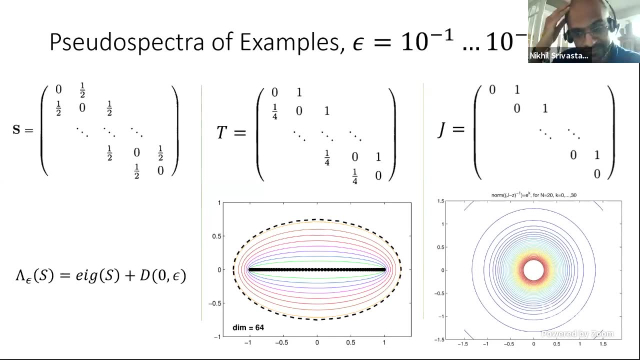 of norm epsilon. So that's the pseudo spectrum. So let's look at our three examples in terms of pseudo spectrum. So the first matrix is emission. The pseudo spectrum is literally just a disk of radius epsilon around the spectrum Boring. If you look at P, the pseudo spectrum is a lot more interesting. 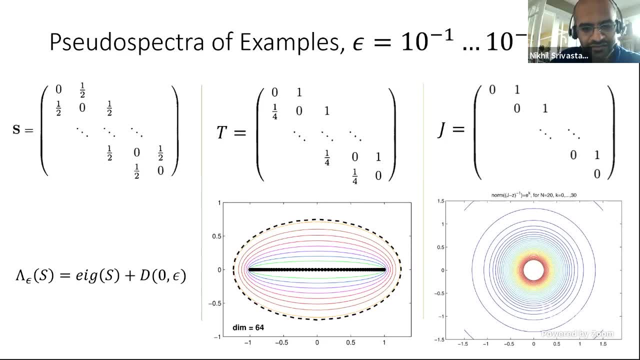 So the black dots are the eigenvalues And these curves are the level curves of this function, the norm of the resolvent For epsilon, I believe, going down from 10 to the minus 1 to 10 to the minus 16.. 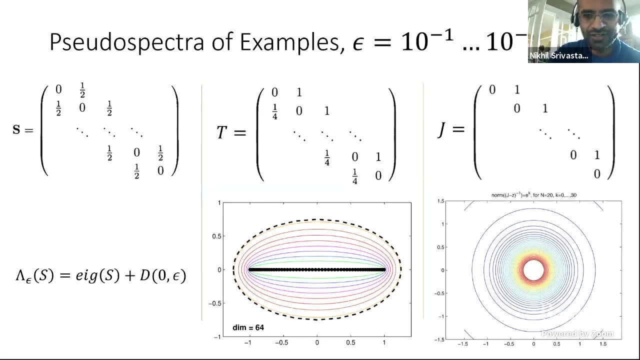 So what you see. so the outermost curve is the 10 to the minus 1 pseudo spectrum. So if you had a perturbation of size of 10, the eigenvalues can travel that far And notice that that's a lot bigger than a 10.. 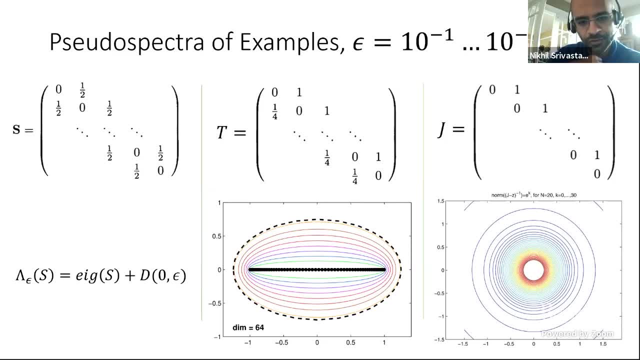 But even more stark is: look at the inner pseudo spectra right. So the innermost oval or whatever shape that is, is a 10 to the minus 16 pseudo spectrum. So you're adding perturbation of size 10 to the minus 16 to the matrix. yet the eigenvalues. 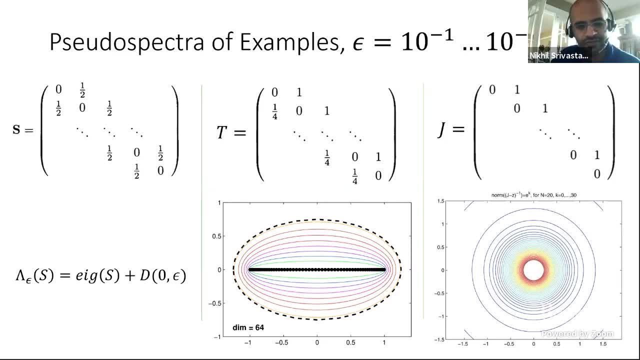 can move macroscopically far away. So this really is what we mean by spectral instability: that the spectrum moves a lot when you add a tiny perturbation. Then finally, for the Jordan block, if you actually plot the pseudo spectrum you get. 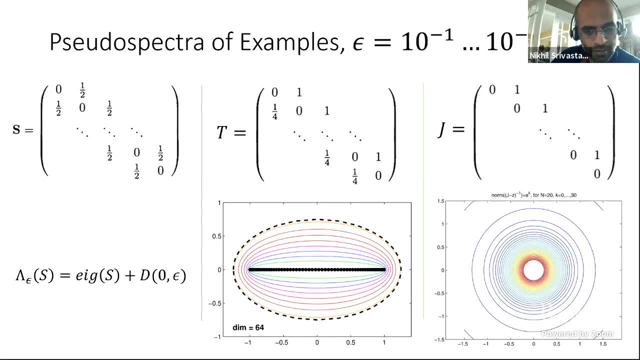 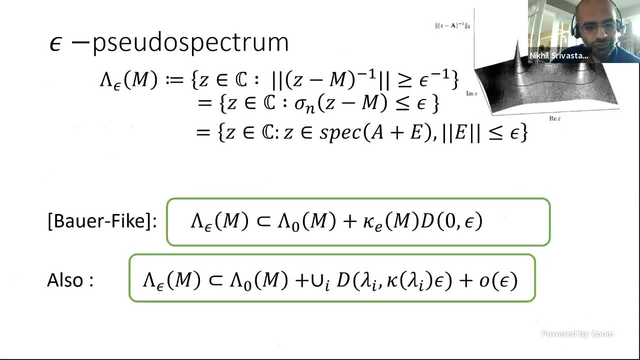 some even bigger disks. OK, So the pseudo spectrum. The pseudo spectrum is now a third notion of spectral stability that I'm going to relate to my previous two notions. So the Bauer-Feig theorem says that the pseudo spectrum of a matrix is contained in disks. 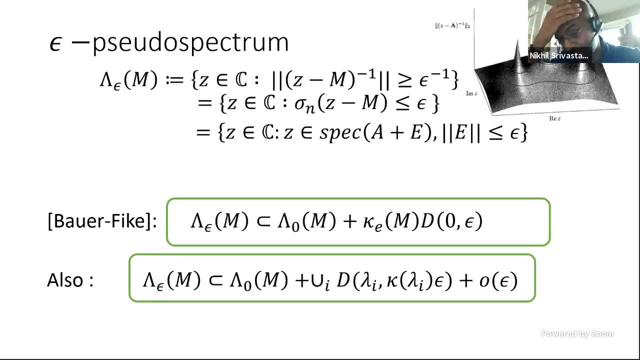 of radius, at most the eigenvector condition number around the eigenvalues. So this means if you have small eigenvector condition number, you have small pseudo spectrum And similarly if you have small eigenvalue condition numbers. so these kappa lambda i. 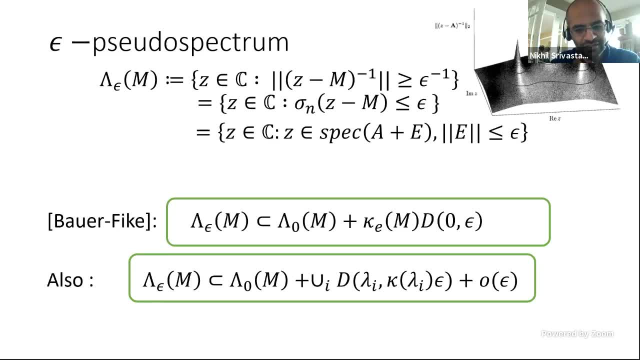 then the pseudo spectrum is contained in disks of radius about kappa lambda i epsilon times the i-th centered at the i-th eigenvalue in the regime of small, very small perturbation, epsilon. OK, So high level if you control the previous, any of either of the previous two quantities. 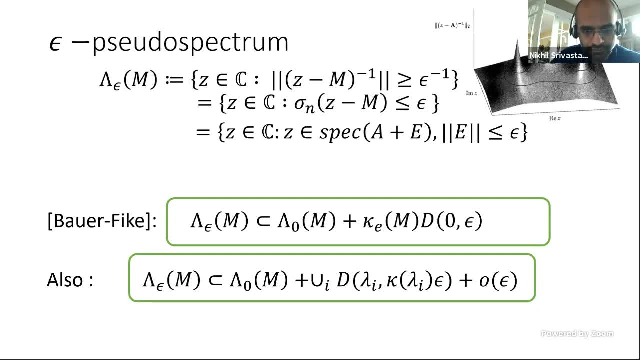 that implies that the pseudo spectrum is small. So any questions about the definition of pseudo spectrum or any of these equivalences? No, OK, So I've introduced three Mm-hmm. Maybe a question of computability. Vince mentioned numerical linear algebra. 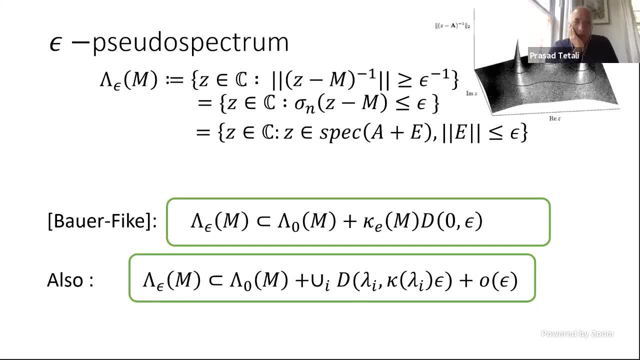 How easy is it to work with pseudo spectrum? How easy is it to compute? I don't know. off the top of my head, There are algorithms, There are MATLAB packages that do it. I don't know if people, computer scientists, have seriously studied the complexity of doing. 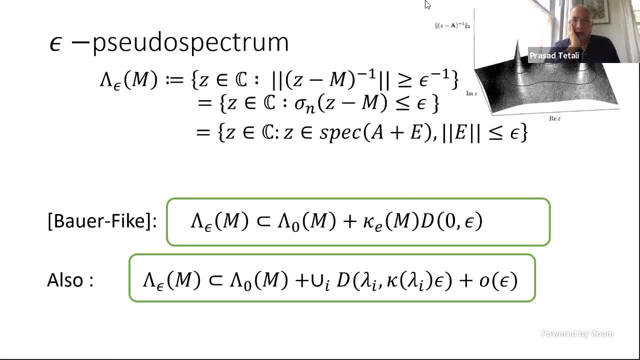 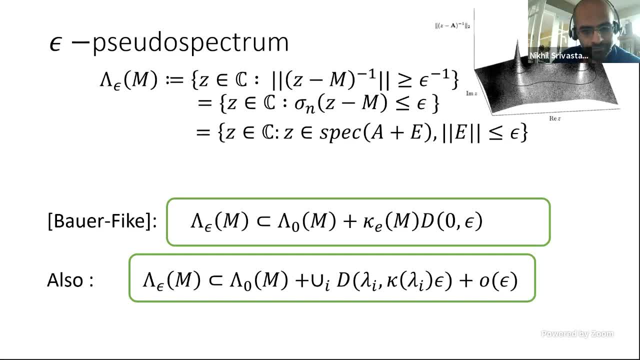 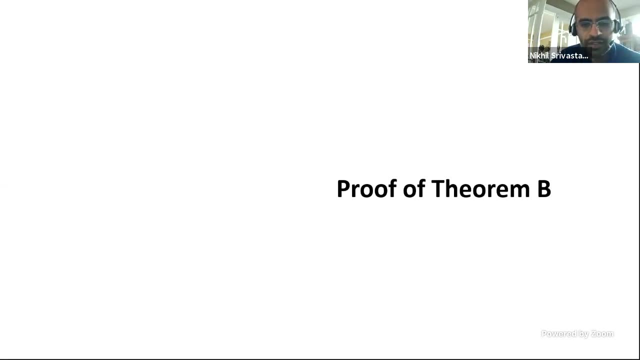 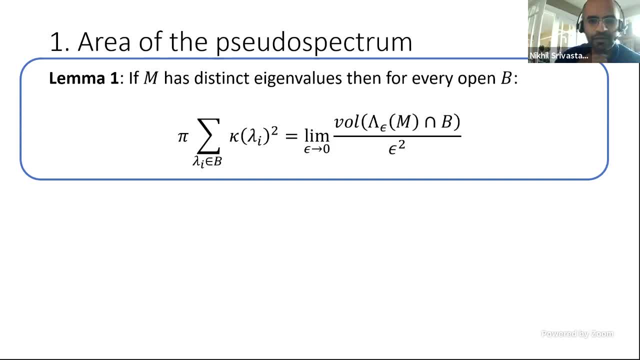 area of the pseudo spectrum. okay, so here's lemma one. it says: if you have a matrix is a deterministic lemma about every matrix. if you have a square matrix with distinct eigenvalues m and you have some open set b, then the sum of squares of the eigenvalue condition numbers of the eigenvalues in that. 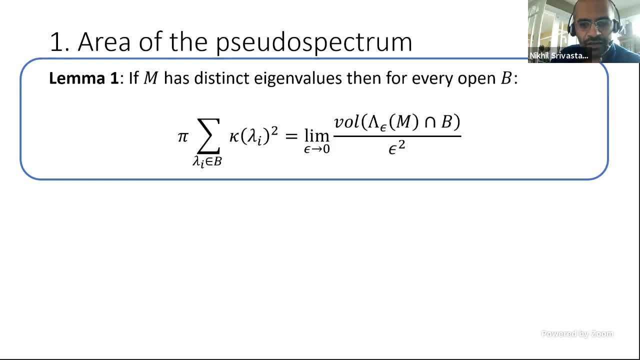 set. this is equal to the limiting area of the epsilon pseudo spectrum restricted to that set, as divided by epsilon, squared as epsilon goes to zero. okay, so i'm writing this as a scaling limit of the area of the pseudo spectrum. okay, so this is not a new lemma. this is, uh, must be have been known for decades. here's uh, but what? 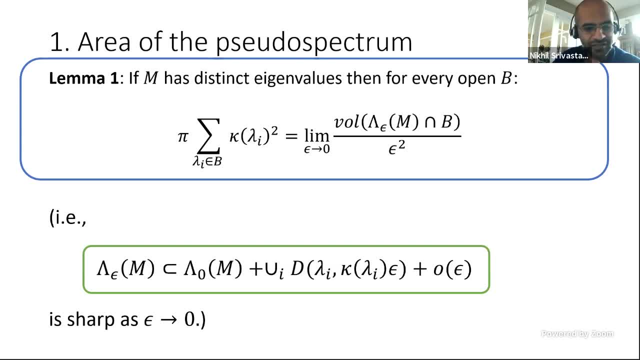 it says is that there's a converse to the fact that i wrote on the previous slide. so in the previous slide i wrote that the epsilon pseudo spectrum is contained in disks of radius of kappa lambda i times epsilon around the eigenvalues lambda i. well, if that was actually. 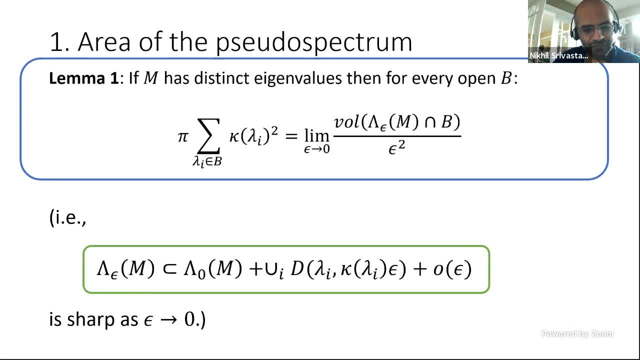 sharp. well then the area. what would be the area of the pseudo spectrum? it would just be, you know, pi times kappa lambda, i squared times epsilon squared, the sum of those quantities. so if you divide by epsilon squared, you would get the quantity on the left hand side. 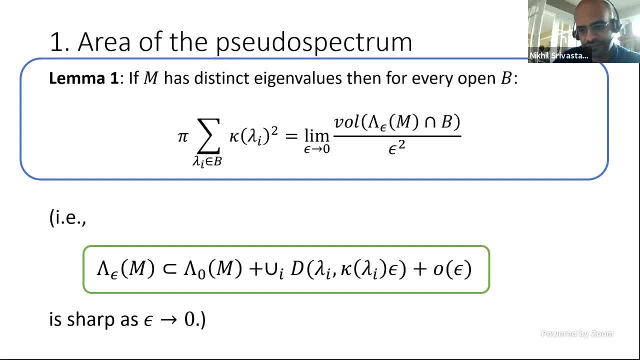 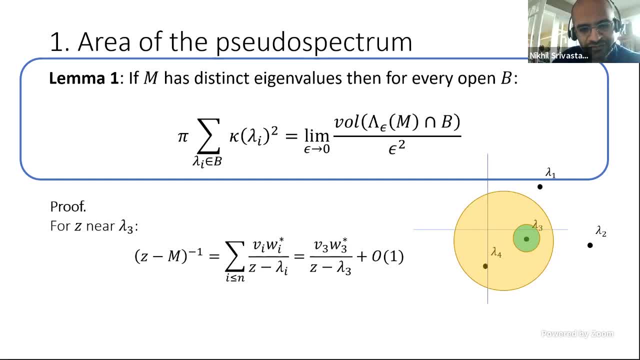 and you take the spectral expansion of the resolvent and let's suppose you have some number z that's close to some eigenvalue, let's say lambda three. well, as you approach the eigenvalue, all the other terms become, are bounded right. the only one term is blowing up. 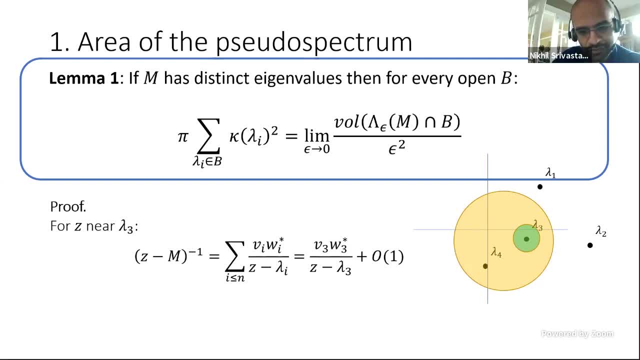 the one corresponding to the eigenvalue lambda three. so you have this v3w3 star, that's the spectral projector onto that subspace, divided by z minus lambda three, plus something that's bounded as z approaches lambda three. so then that's the eigenvalue of lambda three. so then, 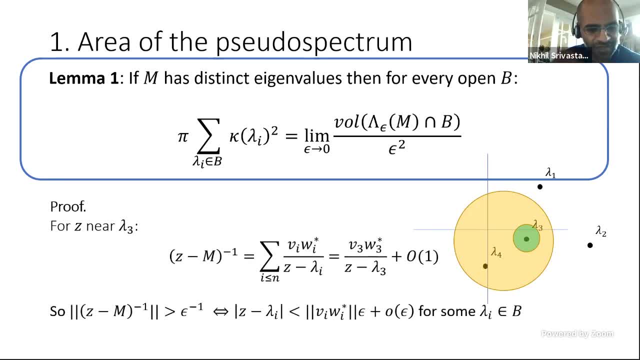 that's it right now. you just see it. so in the regime of very small epsilon, the resolvent being bigger than one over epsilon implies that for some eigenvalue this term has to be bigger than one over epsilon, and that's the same thing as saying that z is within distance. uh, the norm of 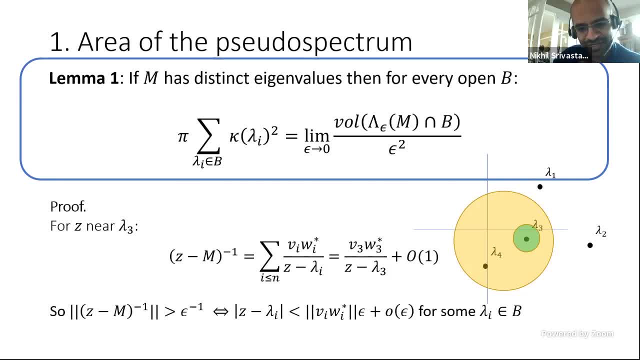 the spectral projector times epsilon of some eigenvalue, but that's just the norm of the spectral projector is just the eigenvalue condition number. okay, so this is like a one-line proof. basically, it's just a one-line proof. so you can see that it's just a one-line proof, so you can. 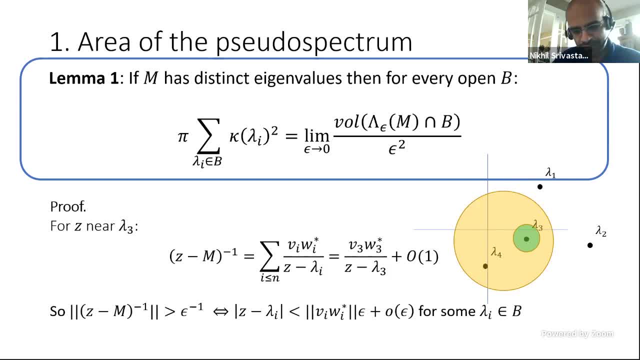 see that it's just a one-line proof. basically, when you go near an eigenvalue, the matrix becomes rank one, and for rank one matrices this is kind of obvious, okay, so any questions about this lemma? so what i'm doing is i'm passing from the eigenvalue condition numbers to area of the. 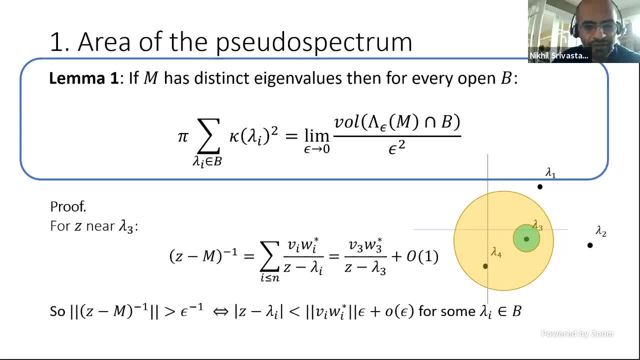 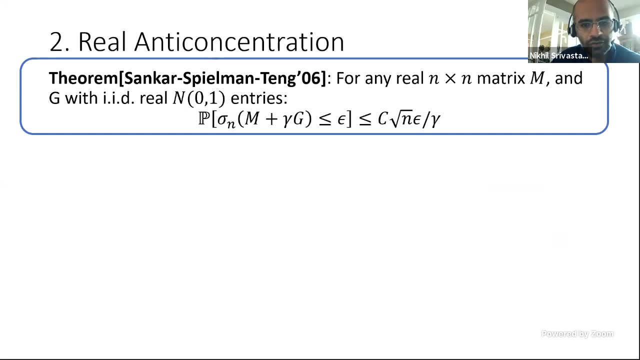 pseudo spectrum. and okay, why not, for fun, just throw in lim inf here. that'll be useful later, okay, so now my goal becomes to control the area of the pseudo spectrum. so how would i do that? well, the main tool i need to do this is comes from smoothed analysis. 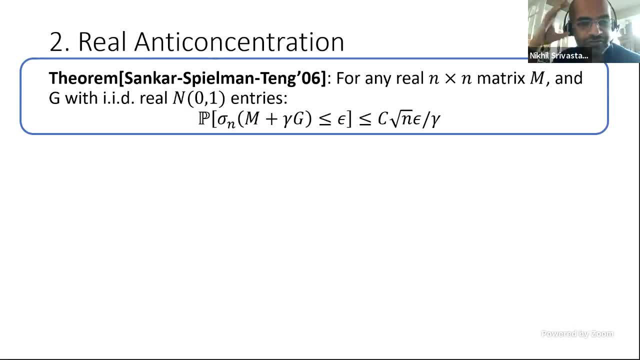 uh, and it's. it's the following: uh, the starting point is the following: theorem of sunkers, spielman and tang, which says: if you take any real n by n matrix and you add a gaussian with real independent, with iid, real standard gaussian entries, then the probability that the least 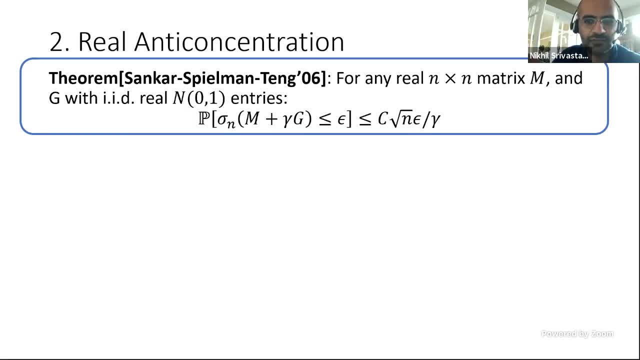 singular value of m plus gamma g. so that's why it's a smooth analysis. you perturb the fixed matrix by this random matrix probability. that that has a least singular value. less than epsilon is some constant times squared n times epsilon over gamma. okay, so it makes sense that. 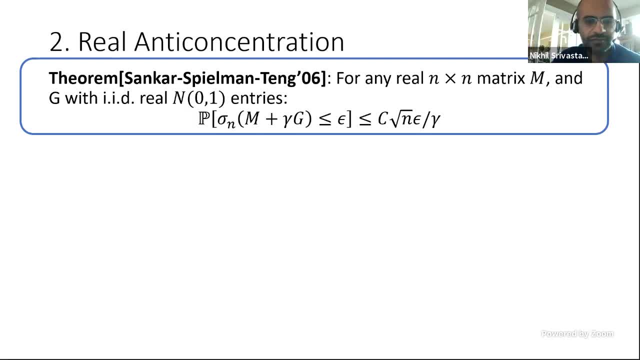 this bound should get worse as gamma gets smaller. if you take a bigger perturbation, you expect more regularization. um, and the you know maybe important. so the important feature of this bound is that this decays as the probability that the least singular value is less than epsilon decays as epsilon. 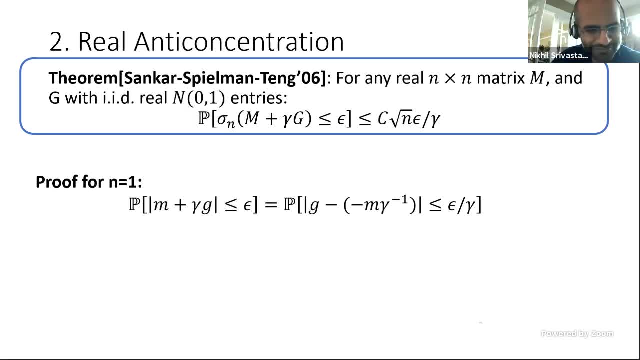 so what's the proof of this? let me prove this in: n equals one. okay, so for n equals one, m is a number, gamma g is a number. the probability, the least singular value, is just the magnitude of the number, the probability that m plus gamma g is less than epsilon. so epsilon is some fixed, some fixed. 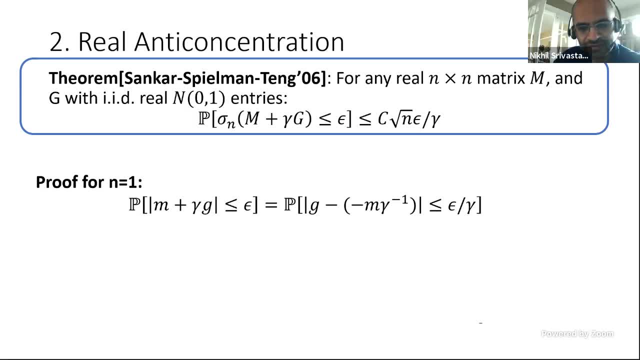 parameter. this is just equal to the probability that the standard gaussian g is within distance epsilon over gamma of minus. that's just literally what it is. and then by some very standard anticoncentration, this is at most m epsilon over gamma. the gaussian, you know, the most mass it puts is on the window near zero, and you just get that. it's this. 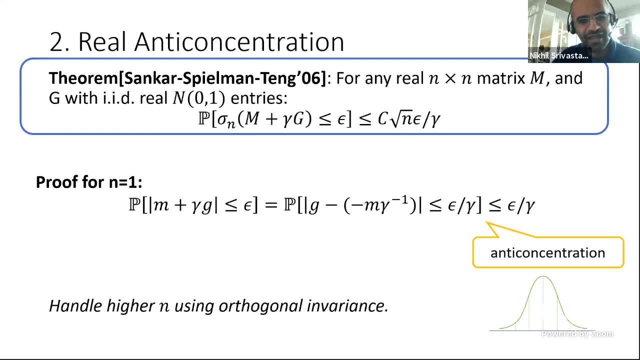 so, of course, the proof for matrices is more complicated. at a high level they handle this using orthogonal invariance, but this is the thing i want to emphasize about. the proof is that the dependence on epsilon comes from comes from this one dimensional factor, Paraf—. 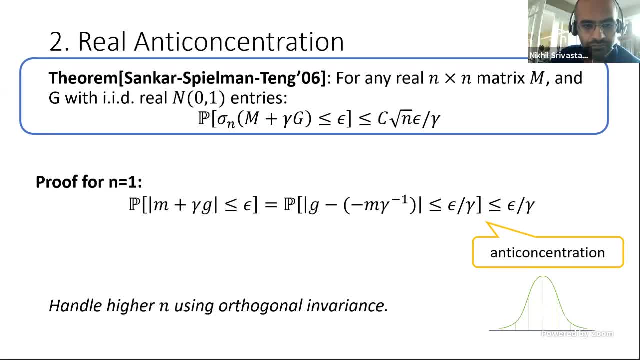 about anti-concentration of real Gaussians And what is known about the reverse inequality. Well, when m is 0, the reverse inequality is No, but I mean for various m, I don't know. I mean, is there any result? 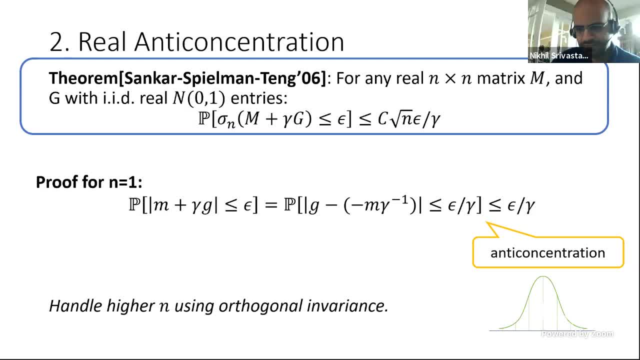 I mean. so I think there are results. I don't know if there is a crisp conjectured lower bound in terms of some function of m. I think Vishesh might know more about this than I do, or maybe his co-authors. 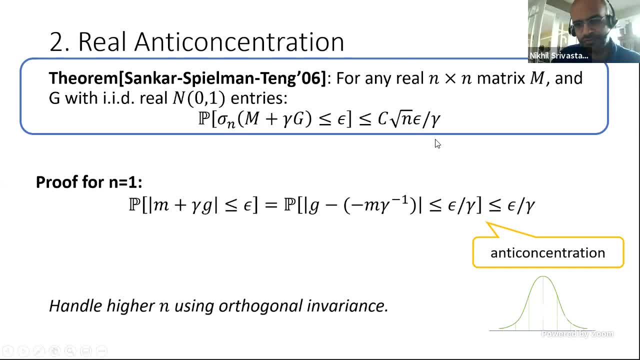 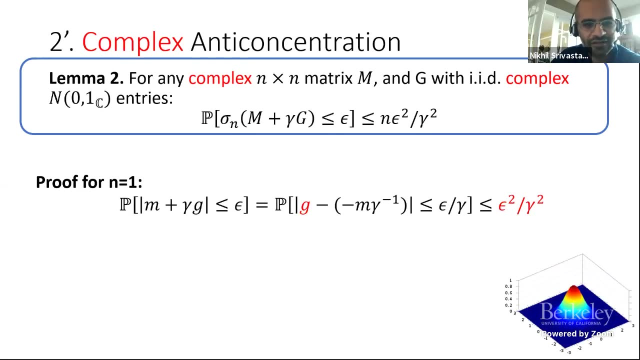 But I don't think there's a very crisp characterization of how this bound depends on m. OK, so the second step in the proof is not this, but it's a variation of this. It's well, what if you take a matrix and add a complex Gaussian? 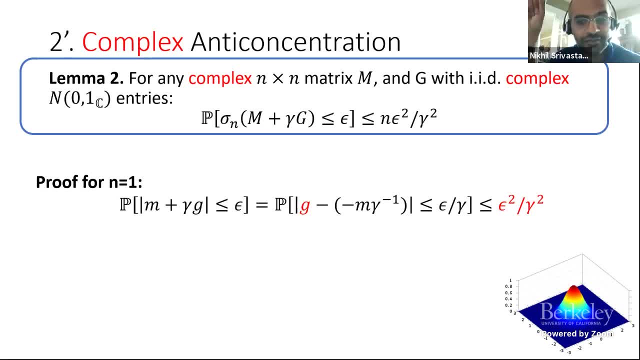 So this is lemma 2.. So you take any Gaussian, You take any complex matrix and add a matrix with complex iid Gaussian entries. So then the claim is that the probability that the least singular value is less than epsilon decays as epsilon squared over gamma squared. 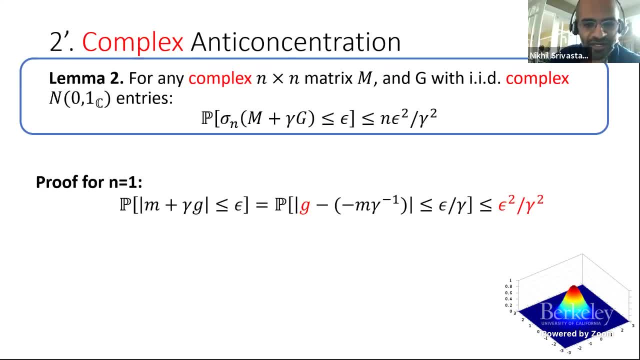 So everything gets squared. Now, what's the proof for n equals 1?? Well, the same. you know, it's the probability that a complex Gaussian is close to some fixed number. But now, this is the whole point, that the complex Gaussian 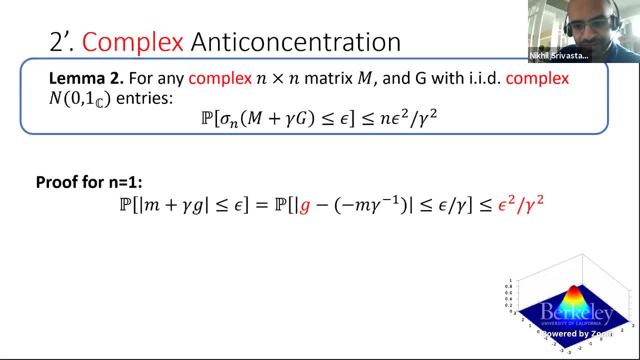 is a two-dimensional object, So the probability that it's close to any point in the complex plane decays is the square of the distance to that point. So you get epsilon squared over gamma squared, And so, OK, the way we actually prove the lemma for matrices. 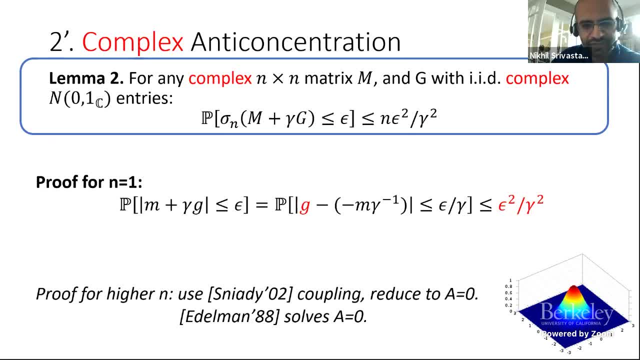 is we use a coupling theorem of to reduce to the case of a equals 0. And then the case a equals 0 is exactly solved by Edelman of the 80s. OK, so the thing I want to emphasize is: you go from epsilon to epsilon squared. 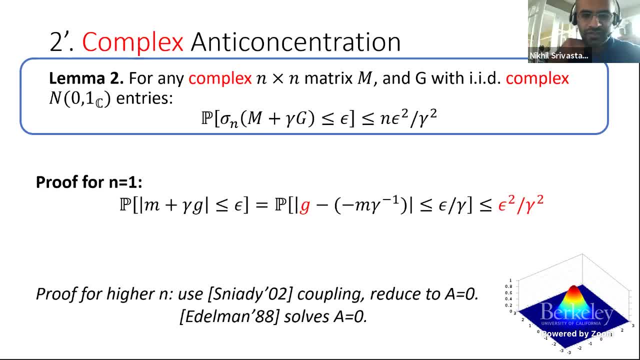 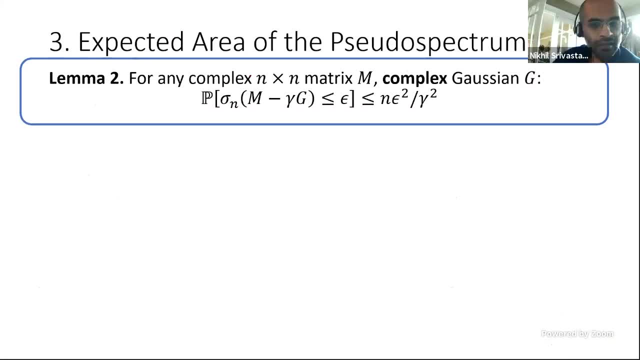 when you take a complex Gaussian. OK, that's step two. Now step three is to use this To control the area of the pseudo spectrum in a sort of obvious way. So lemma two says that if you take any matrix m and subtract gamma g from it, the probability 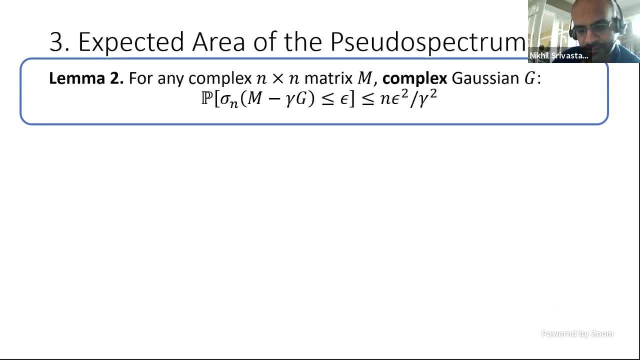 that at least singular value is less than epsilon decays as epsilon squared over gamma squared. So now let's apply this to a shift of my input matrix a. So remember, in the background there's this input matrix a that's given to me. 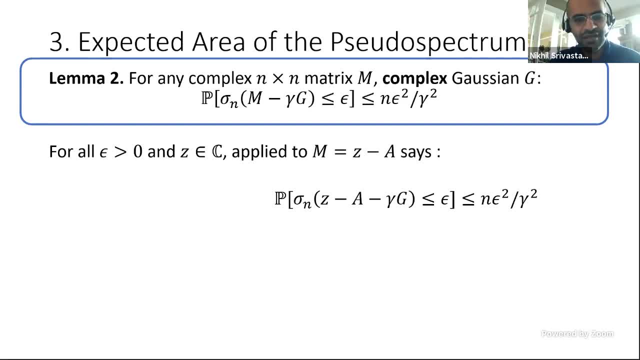 So let's fix some epsilon, fix some complex number z and look at z minus a, the shifted matrix. Well, the theorem says that the probability of the least singular value of z minus a, minus gamma g is less than epsilon is upper bounded. 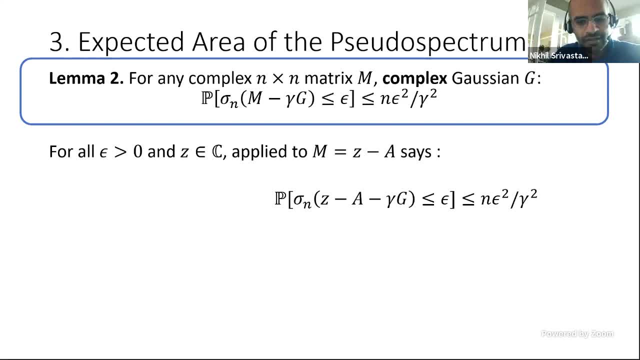 by this quantity, epsilon squared over gamma squared, But that's literally the probability that z is in the epsilon pseudo spectrum right? That's the definition of pseudo spectrum. So what I actually have shown is that for every complex number and every epsilon, the probability 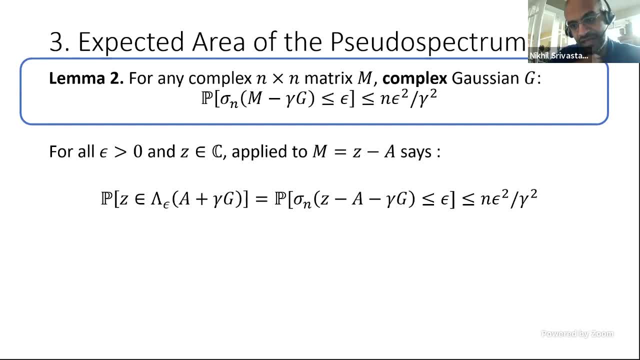 that that number falls in the epsilon pseudo spectrum has this kind of decay. OK, But that's very nice, right? Because if you fix some ball b, well what's the expected area of the pseudo spectrum restricted to that ball? Well, it's just an expectation of an integral, of an indicator. 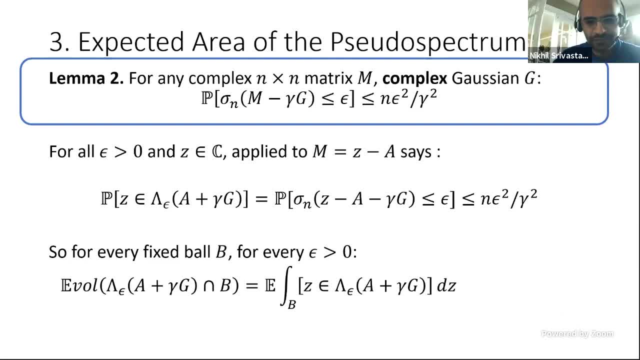 around a variable right. So I just integrate over z in the ball. What's that? z is in the pseudo spectrum. But now I can do Fubini right, So I move the expectation inside. I just need to integrate this probability that a fixed z is. 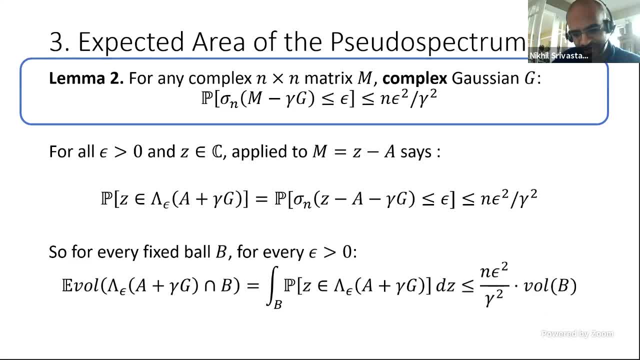 in this epsilon pseudo spectrum. But now I have this like worst case bound on this Right. I just have that for every z It's at most n epsilon squared over gamma squared So quite easily just by this Fubini argument. 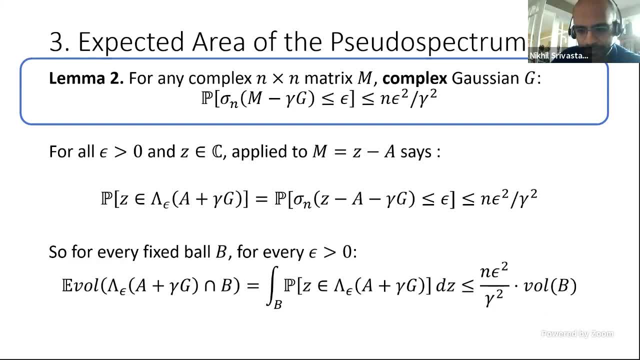 I've computed the expected area of the pseudo spectrum And I've upper bounded it by some nice function times: epsilon squared. That's the third step of the proof. Any questions about this step? OK, And then the fourth step of the proof is: so let's call this: 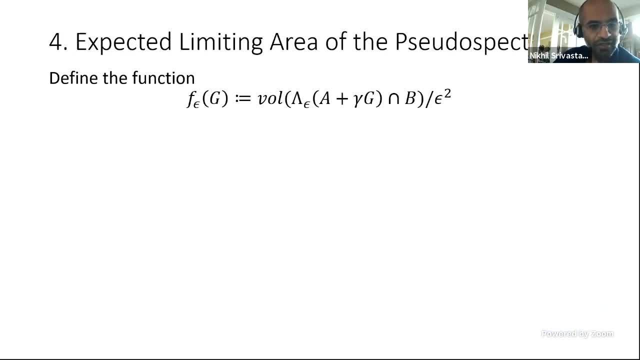 lemma three: For every ball, the expected area is small. And then lemma four, to be very pedantic, let's define a non-negative function which is the scaled area of the epsilon pseudo spectrum by epsilon squared. And lemma three shows that the lim-inf of the expectation 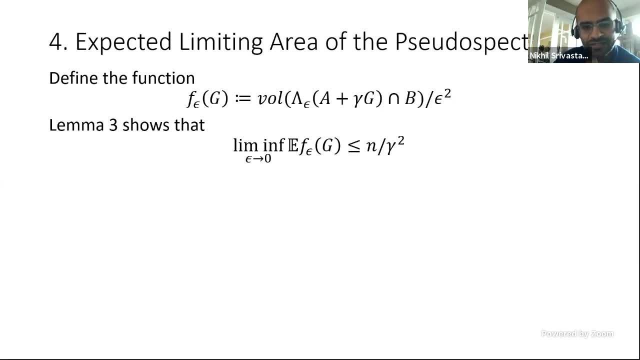 of this is bounded by n over gamma squared right. So I bounded the expected area. So I have that the limit of the expected area is bounded by n over gamma squared, But then by Fatu's lemma that means that the expected limit is bounded by n over gamma squared. 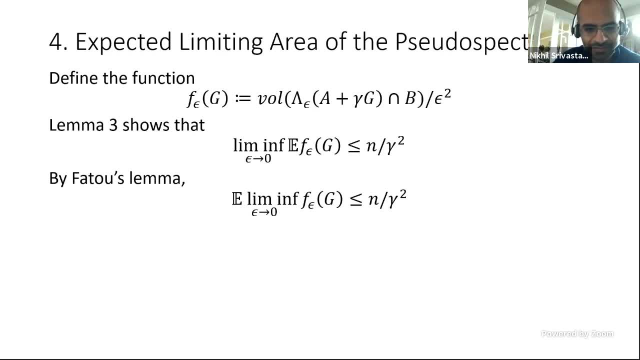 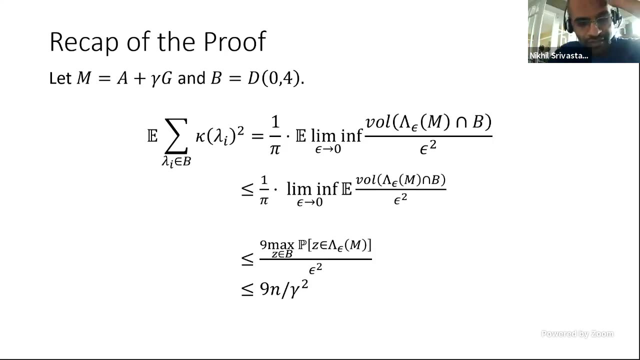 But now, what was lemma one? Well, the expected limit is the sum of squares of the eigenvalue condition numbers times pi. So that's the proof. That's the whole proof. It's very simple. So, to summarize the proof in one slide, this is the proof. 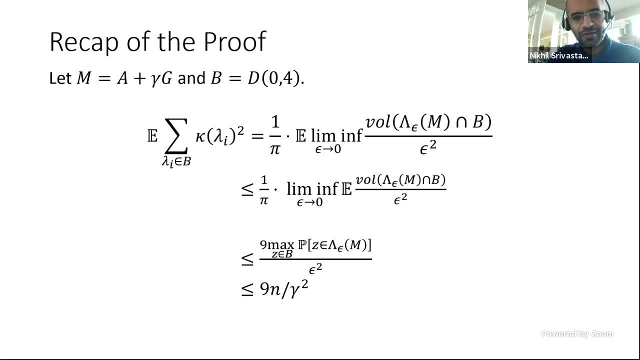 The sum of squares of the expected eigenvalue condition numbers is an expected scaled limit of the pseudo spectrum area which is bounded by the limit of the expected pseudo spectral area Which, by Fubini, can be controlled by just controlling this one tail probability of a fixed point being. 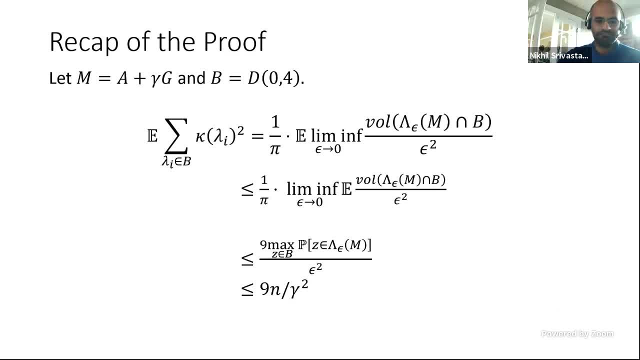 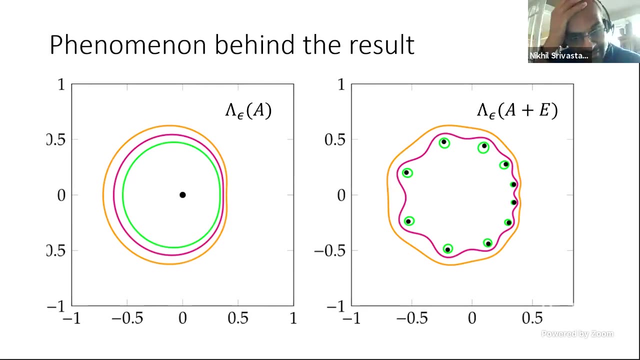 in the epsilon pseudo spectrum which I'm able to produce. So it basically involves changing order of limit and summation three times. So that's the proof of the theorem And this is a picture explaining the mechanism behind the results. On the left-hand side I have a matrix A. 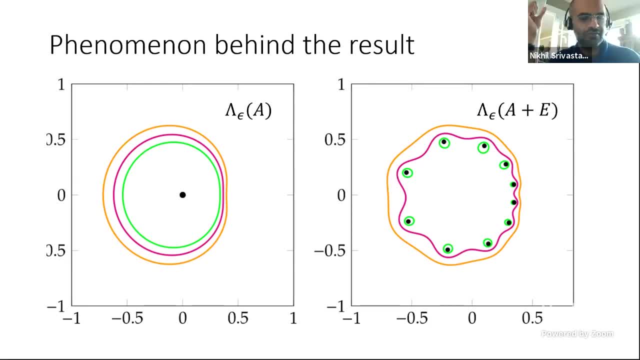 which is quite spectrally unstable. It's actually a Toplitz matrix with all eigenvalues at zero And, as you can see, these are various pseudo spectral contours. These are quite large, The pseudo spectrum is big, And if you add a tiny Gaussian perturbation to it, 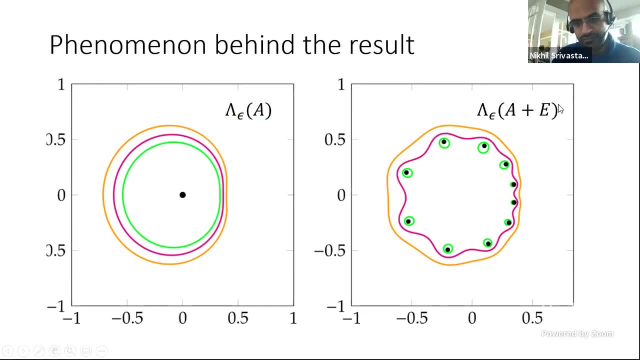 what you get is a picture on the right. So the eigenvalues move a lot, But the new pseudo spectrum as a set is much smaller. The green circles became tiny now. So that's it. That's the proof of theorem B, So the high level idea. 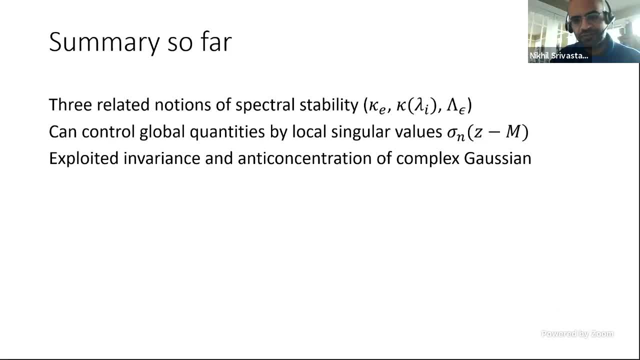 is that it's important to use three of these notions of spectral stability: the eigenvector condition number, the eigenvalue condition numbers and the pseudo spectrum, And by combining these in some appropriate way you can go from a very global quantity such as kappa E. 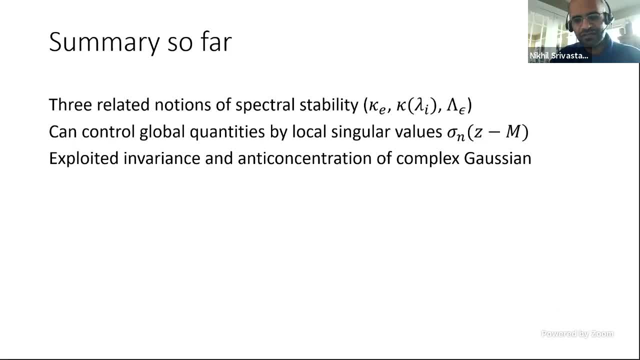 to very local quantities, namely singular values of shifts, which then you can bound using properties of this complex Gaussian. So there's one further development in this, which is something somebody asked about, which is we really heavily use: that the Gaussian is complex. 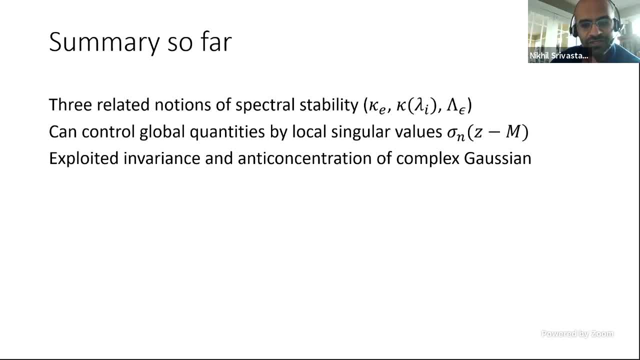 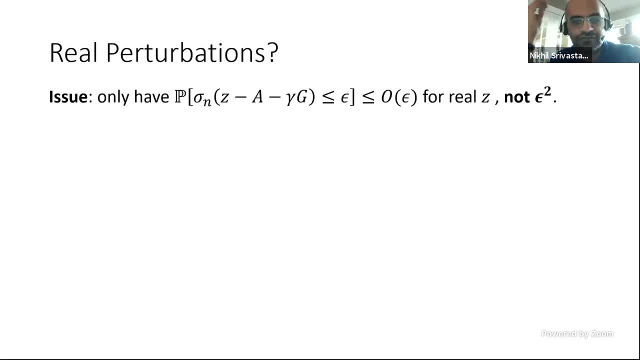 So we use it because you really needed the pseudo spectral area to decay as epsilon squared. So what happens for real perturbations? So if you take a matrix and add a real perturbation, then actually the tail bound you get is only order epsilon. 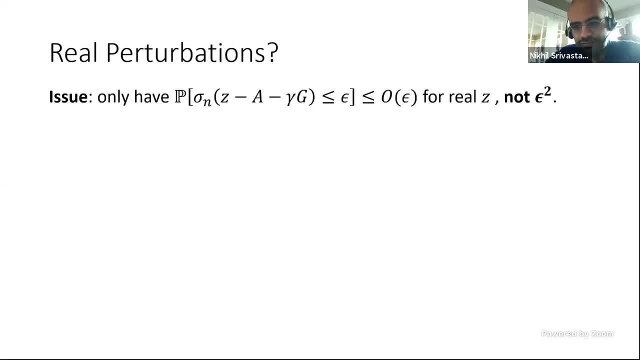 It's not epsilon squared, So you cannot do this argument for real perturbations. The limit will simply blow up. So it's a mystery for a little while whether this can work for real perturbations. But then it turns out there's actually. 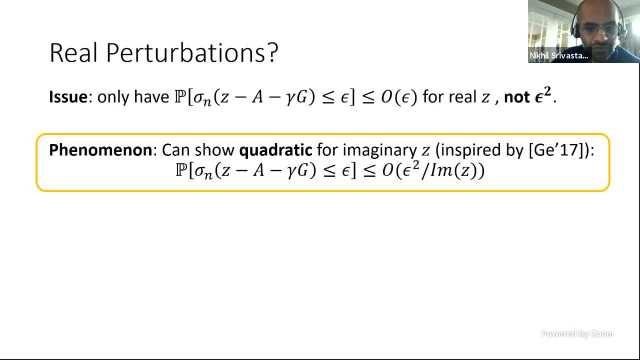 an important phenomenon. that causes this to also work for real perturbations. So what we can show is that, while it's true that this singular value decay is order epsilon for real z, if you have a real Gaussian matrix g and a complex number z, OK, 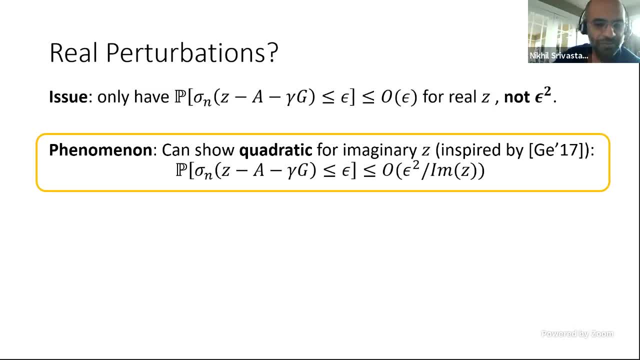 OK, The probability of the least singular value of z minus a, minus gamma g, is less than epsilon. This decays at epsilon, squared over the imaginary part of z. So this is inspired by a theorem that proved in the thesis of Stephen Ge, Where he proved this plus some additive term. 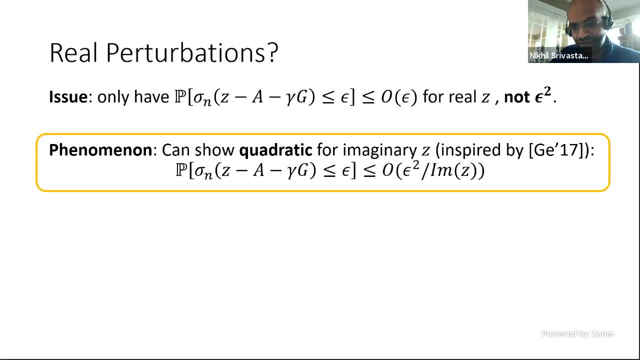 which doesn't depend on epsilon, which was a problem for us. But there's this very interesting phenomenon which is, if you look at the resolvent of a real random matrix, a real Gaussian random matrix, not centered, if you look at it, at complex numbers, 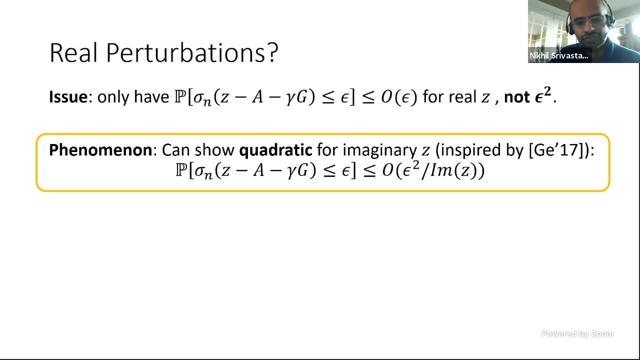 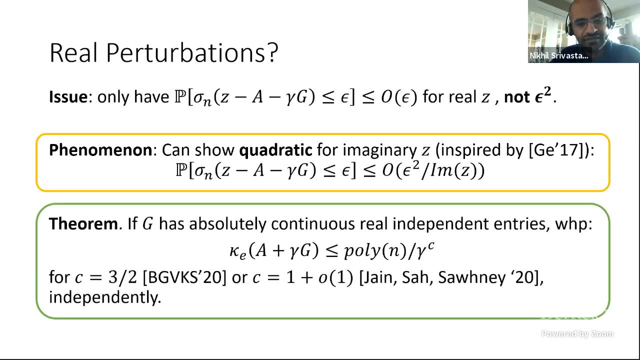 you still get this epsilon squared tail decay. So using this, by proving splitting into real and imaginary eigenvalues, we were able to prove a slightly weaker theorem as theorem A, which is that even for any g with absolutely continuous real, independent entries, the eigenvector condition number 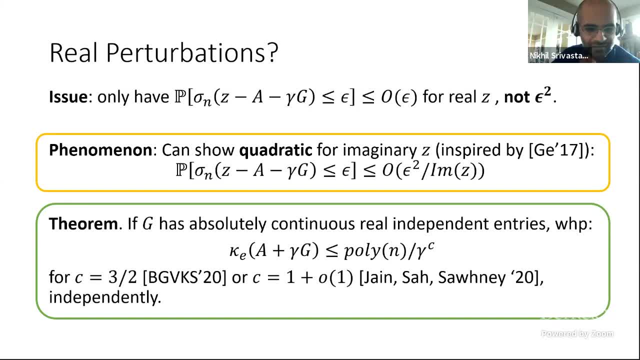 is bounded by some poly n over gamma to the c And we were able to get 3 halves, so not 1.. But independently, j and psi And Sonny proved a stronger result where they're able to get 1 plus little o of 1.. 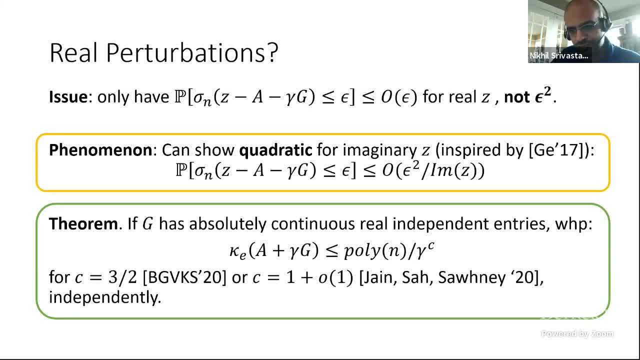 So the conceptual point is that this phenomenon, even though the proof used complex Gaussians, there's a way to do the proof for much more general perturbations. This proof is much more involved, but the phenomenon continues to hold. So I spent more time on that than I wanted. 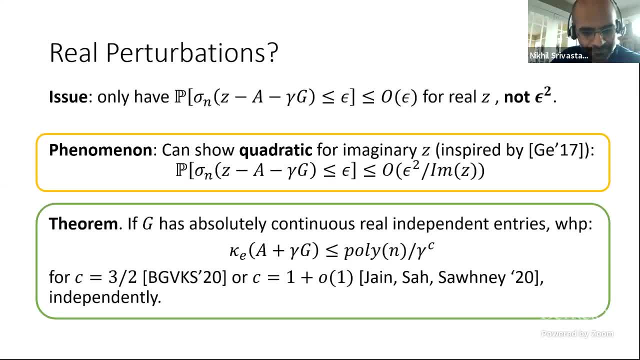 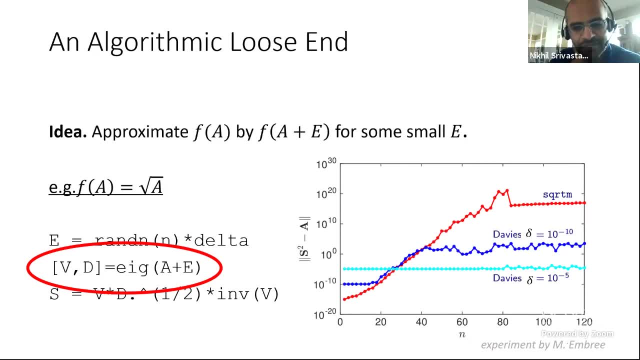 So let me briefly talk about numerical linear algebra for five minutes. So There's actually still a loose end in this story. So in the beginning of the talk I told you that this was my proposal for computing the square root, which is: you give me a matrix. 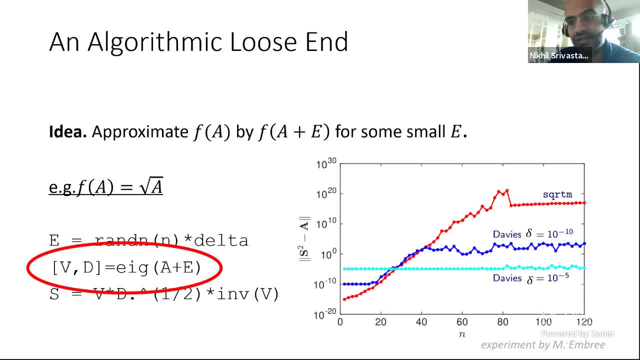 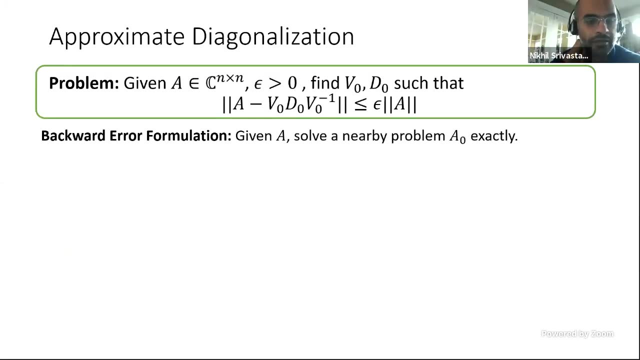 A, I perturb it by random matrix and I diagonalize the perturbed matrix and then I take the square root of that. But how do you actually diagonalize a matrix? So this leads to this algorithmic question of approximate diagonalization, which is a well-defined 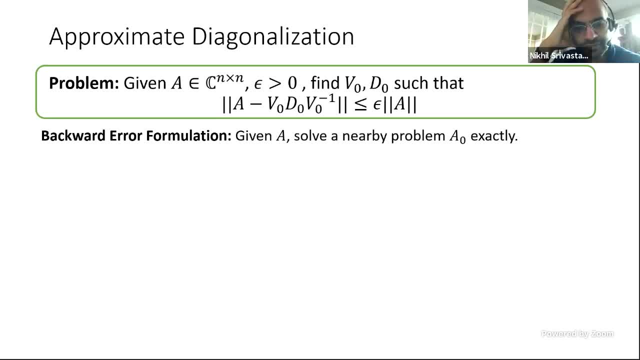 sort of algorithmic question which is given a complex matrix, how do you find its eigenvalues and eigenvectors? So there are many ways of making this formal, And the one that's standard in numerical analysis, which I also sort of argue, is a good one in a moment. 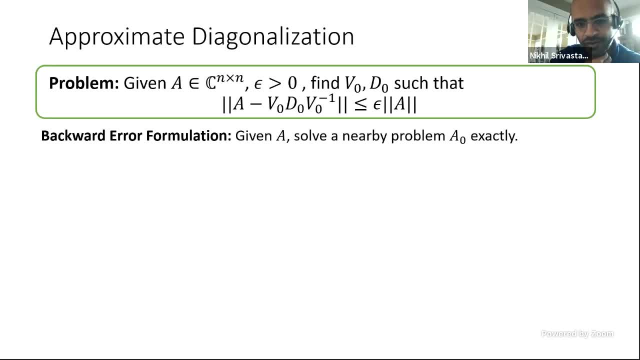 is the following: Given a matrix A and some error parameter epsilon, how do I find some matrices v0 and d0, so that A minus v0, d0, v0 inverse has norm less than epsilon. OK, So conceptually what this is saying is: given an A, 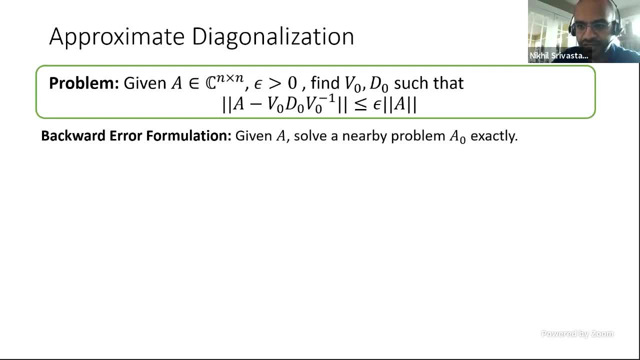 I don't want to compute approximations of the eigenvalues and eigenvectors of A. What I want to do is exactly compute the eigenvectors and eigenvalues of a nearby matrix A0. So this is called backward error and this is a standard notion in numerical analysis. 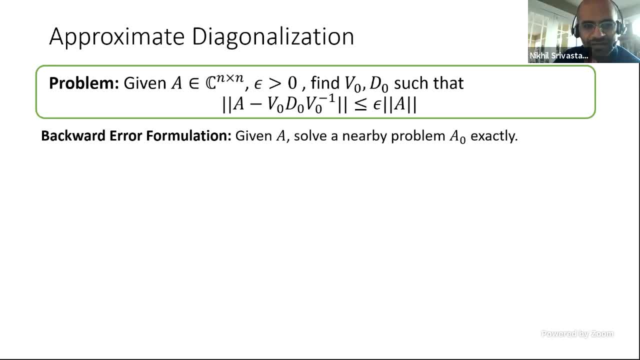 And notice that some notion of error is necessary. right, You cannot compute eigenvalues or eigenvectors of a matrix exactly. on a computer. It's not possible. OK, so that's the problem. And OK, what's the justification for this backward error model? 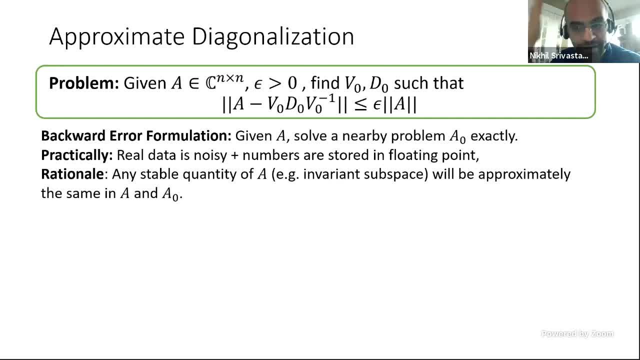 Well, there are two possible ways you could say this is reasonable. One is a very practical answer is that if you're actually doing something on a computer, certainly in scientific computing, if something came from a scientific problem, you never know the matrix exactly in that setting. 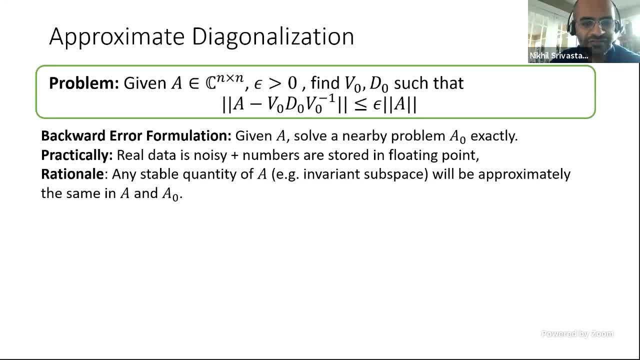 And anyway the numbers are stored in floating point, So you might as well assume there's some tiny error, And so finding an exact answer to a nearby problem is somehow as good as you can hope for. But there's also sort of a deeper mathematical rationale. 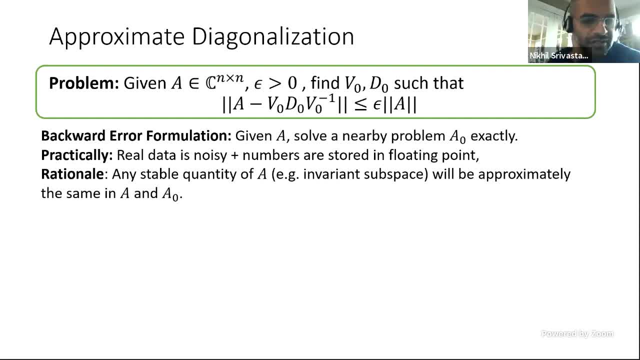 for backward error analysis, which I think is quite beautiful, which is that, well, any stable quantity of any stable feature of A, let's say you want to compute some invariant subspace corresponding to a group of eigenvalues. Or let's say you want to compute an eigenvector. 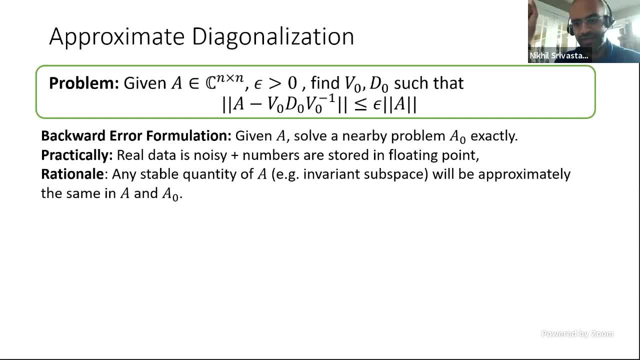 Well, if that quantity is stable- stable means doesn't change drastically under perturbations- well, it's not going to change much when you pass to A0.. So for any stable quantity this is perfectly fine, That the eigenvectors of A0 that you get. 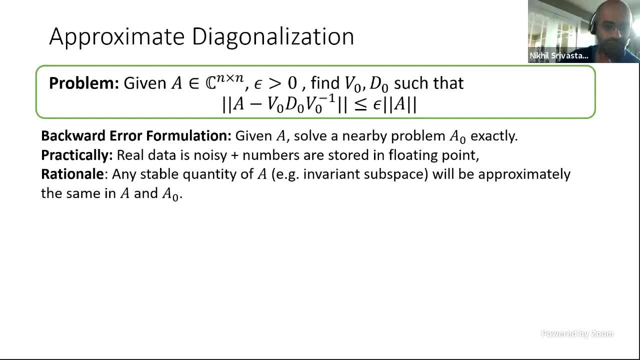 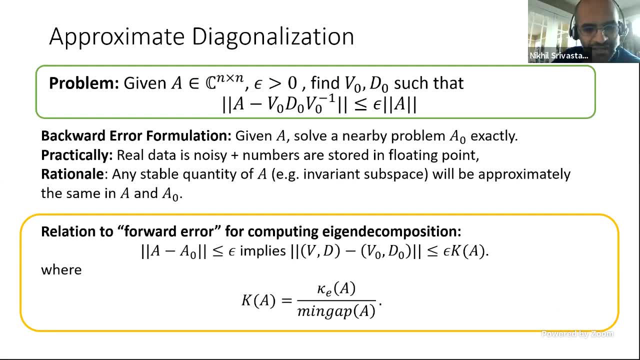 are going to be very close to the eigenvectors of A anyway. OK, So that's backward error. And just to give an example of this rationale, if you wanted to get a forward error estimate given such a backward error solution, the way you would do it is the following: 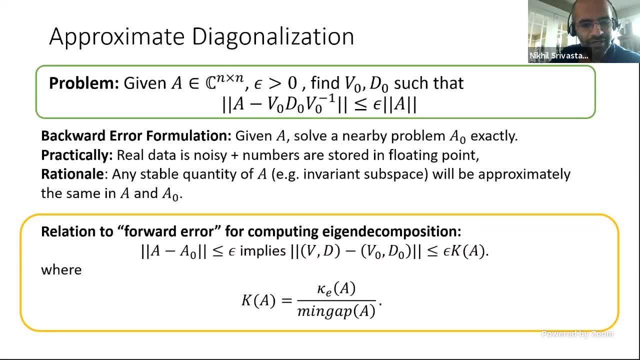 So here's a little theorem: Suppose you have two matrices, A and A0, whose operator norm is differences at most epsilon, Then the distance between their eigen decompositions is bounded by epsilon times. this k of A, which is a new condition number I'm defining which. 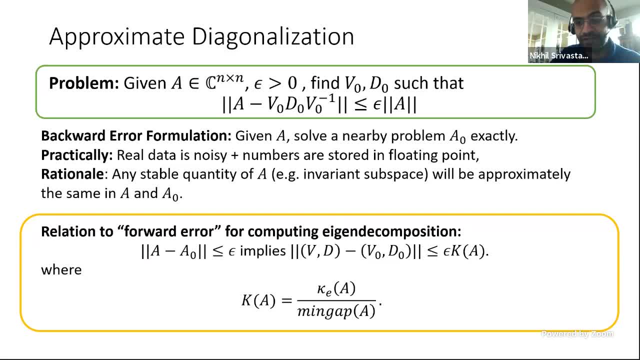 is equal to the eigenvector condition number of A divided by the minimum eigenvalue gap of A. OK, So this is, in particular, this is saying that if you give me a matrix with well-spaced eigenvalues and well-conditioned eigenvectors, 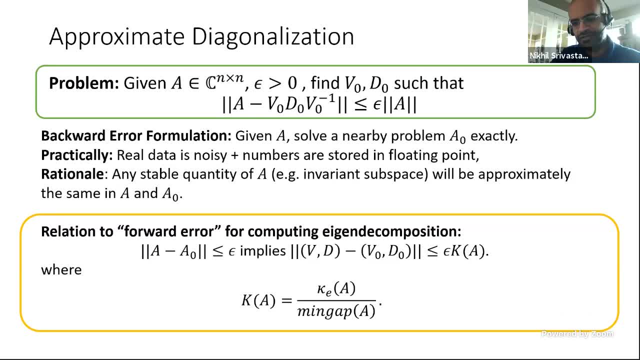 then computing the eigen decomposition of a nearby matrix will give something close to the eigen decomposition of the original matrix. So you can pass from backward error to forward error by arguments like this. OK, So this is the question. So any questions about the question? 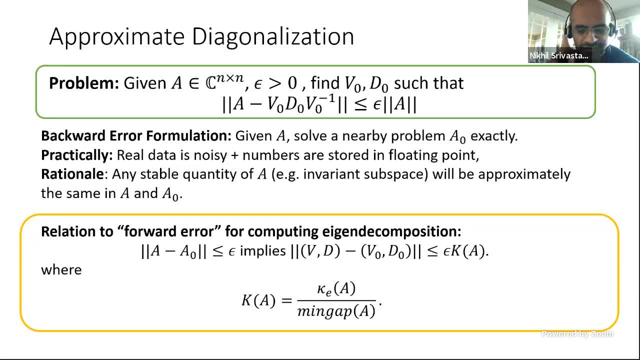 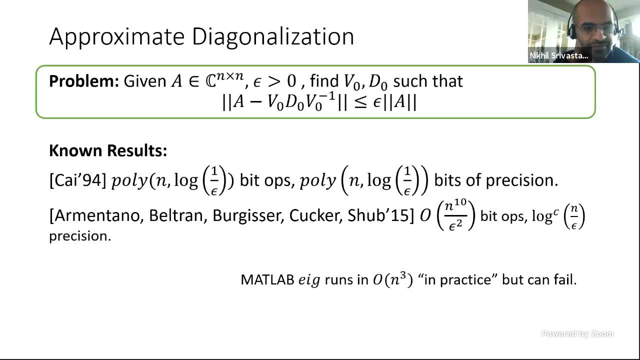 OK, So this is an algorithmic question And, surprisingly, little was known about this question. So this is a quite fundamental question And, as far as I can tell, there are only two rigorous results about this until recently. So the first result is due to Jin-Yi Tsai, from 1994.. 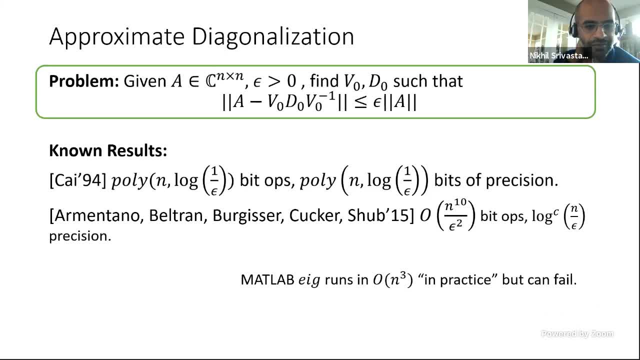 And what he proved is that you can solve this problem in polynomial time. polynomial number of bit operations. OK, So you give me some rational matrix A and you can solve this problem in polynomial time. OK, Then in time polynomial in the length of the input. 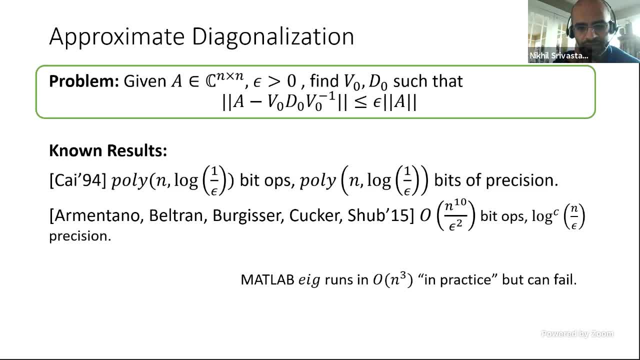 I can produce such a v0 and d0. In time, polynomial in n and log 1 of epsilon, And I need to do this. I need to do arithmetic with numbers of size, polynomial in n and log 1 of epsilon, And these polynomials are quite large. 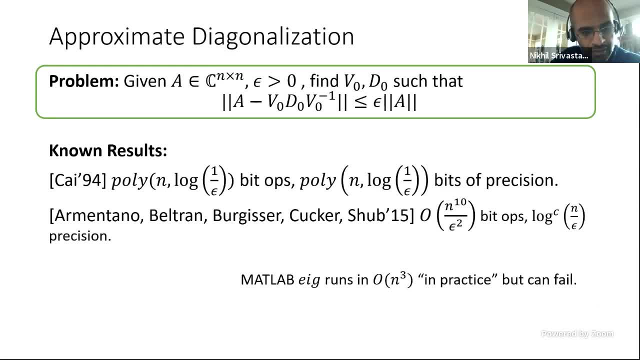 I think the final running time was n to the 12th, So for a while it was an open question about: well, how Is there an algorithm that solves this eigen problem using a small amount of precision, like, ideally, polylogarithmic? 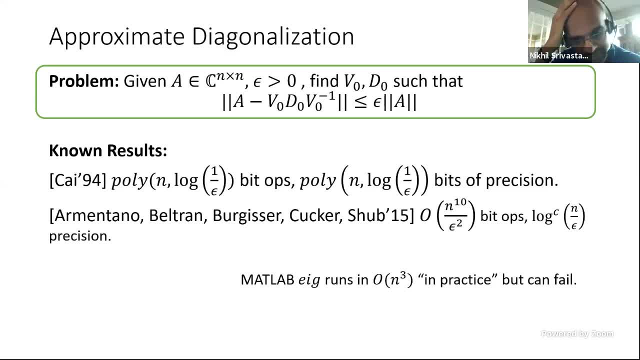 OK, So on an actual computer you don't use polynomial in n bits of precision, So that's called a numerically stable algorithm, And this was open for, I guess, several decades And it was solved at least in a polynomial time. 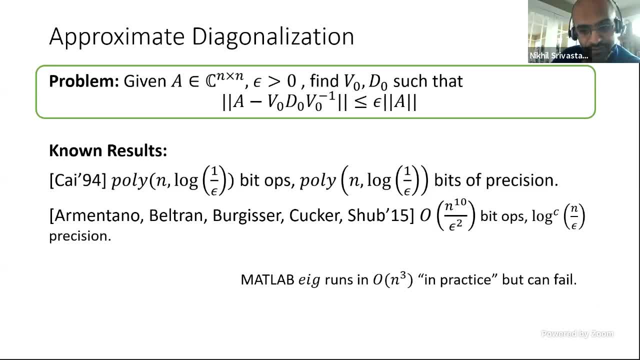 sense by Armentano, Beltran, Bergeser, Cooker and Schubb in 2015.. And they proved that there is an algorithm that solves this problem in time. n to the 10 over epsilon, squared using numbers of Only polylogarithmic bit length. 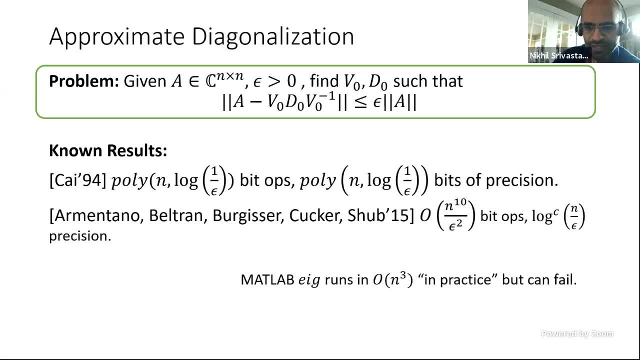 So you might find this surprising, because people run IEG and MATLAB all the time. But IEG is actually just a heuristic, It's not a proven algorithm And there are examples where it doesn't work. MATLAB can actually literally say: I can't diagonalize this matrix. 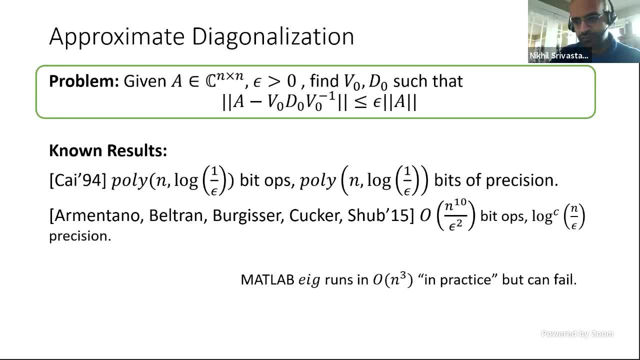 And you might also be surprised because you might think that diagonalization is an n cubed operation. Well, it is n cubed for Hermitian matrices. There's a famous result from the 60s which says that for Hermitian 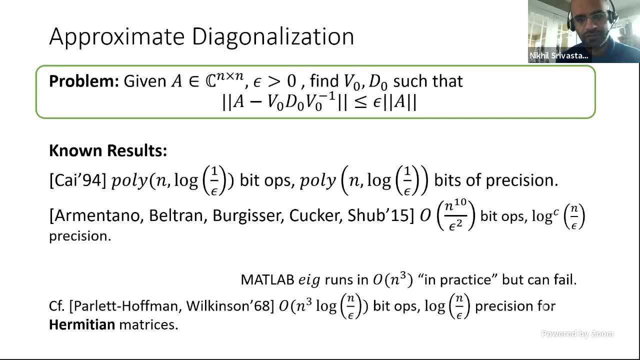 matrices. you can solve this problem in n cubed log n over epsilon operations with logarithmic precision. OK, so this is kind of a loose end. We don't actually have an algorithm for doing this. So the other result I just want to mention. 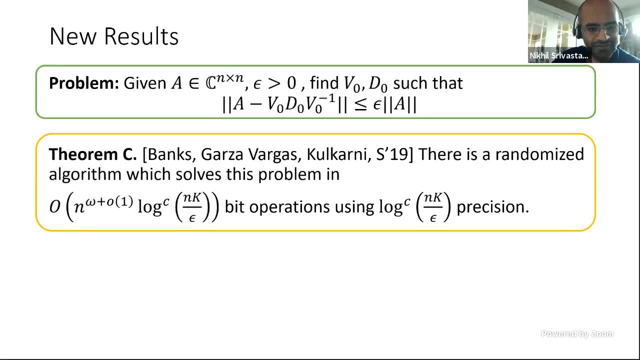 is that we proved this theorem C last year, which is that, yeah, there is a randomized algorithm which actually solves this problem in nearly matrix multiplication time. So it solves the problem, And so omega is exponent of matrix multiplication. It requires n to the omega poly log in nk over epsilon bit. 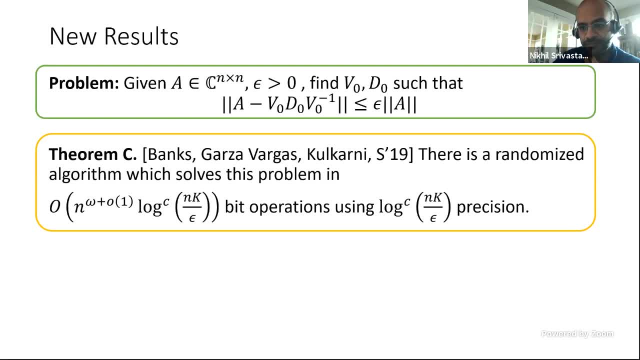 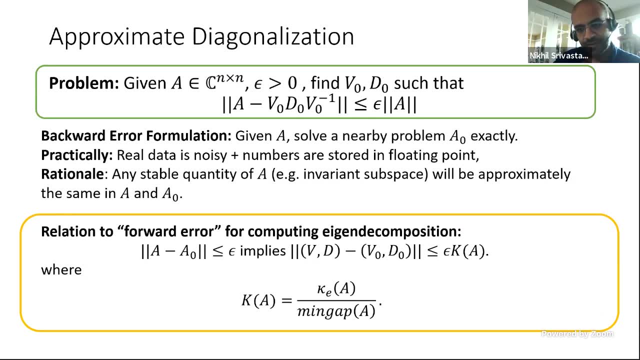 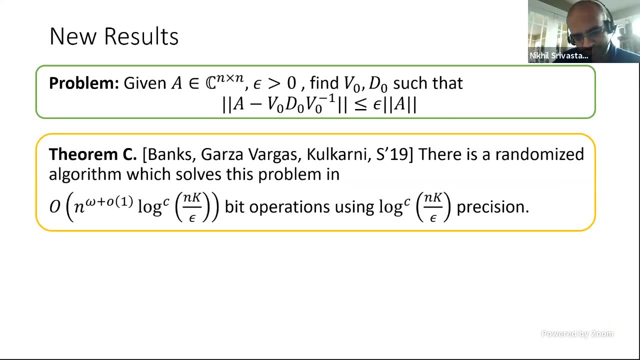 operations using poly log in nk over epsilon precision. Now k is this parameter from a couple of slides ago. It's eigenvector condition number divided by the minimum eigenvalue gap. This is, I guess, quite an improvement over the previous results. 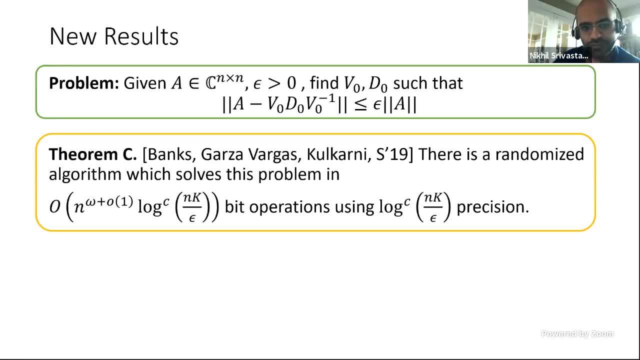 But it still doesn't solve the problem written above. The problem written above is: well, how do I do it for any matrix? This is saying I can solve this problem in logarithm of a certain condition, number, runtime. But what about any matrix? 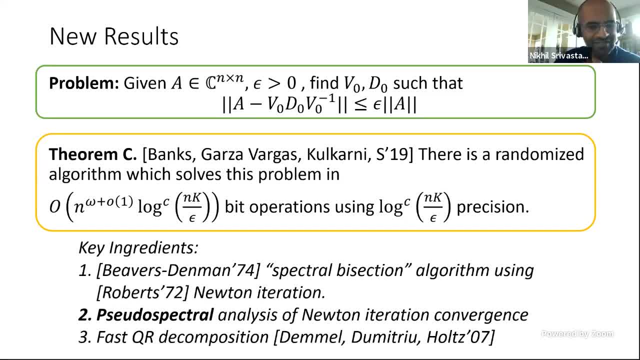 Well, we can. OK, maybe I'll just briefly say: the key ingredient in the proof of this theorem is: this theorem is based on an algorithm that's 50 years old. The algorithm is based on a certain Newton iteration, And what was missing was a proof that that Newton iteration still 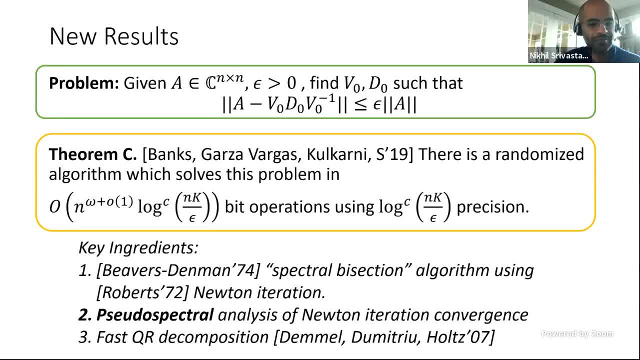 converges In finite arithmetic. So the main contribution of the main technical work in the theorem is a pseudo-spectral analysis of the convergence of this Newton iteration. But anyway, given this theorem, we also proved the theorem A plus, which is sort of an enhancement of the theorem A. 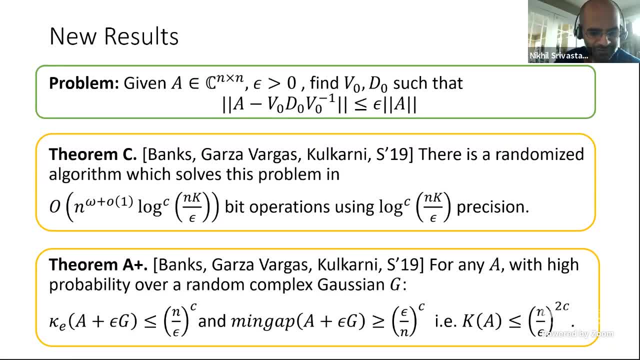 that I gave you earlier which says: if you give me any matrix- and I had a complex Gaussian matrix- then with high probability the eigenvector condition number of the perturbed matrix is bounded by polynomial in n over epsilon And the minimum eigenvalue gap is large. 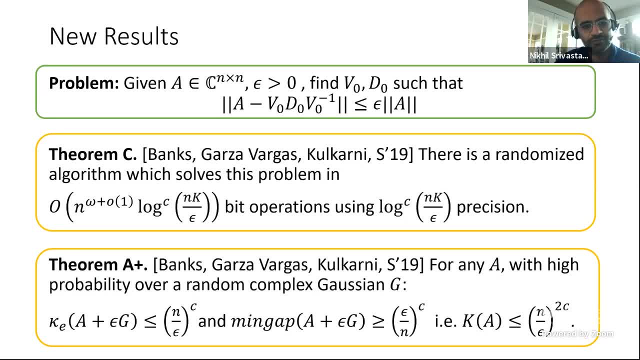 It's larger than epsilon And to some constant. So the perturbation is regularizing in two senses: It makes the eigenvalues move away from each other And it makes the eigenvector condition number small. So given this theorem, it's an immediate corollary. 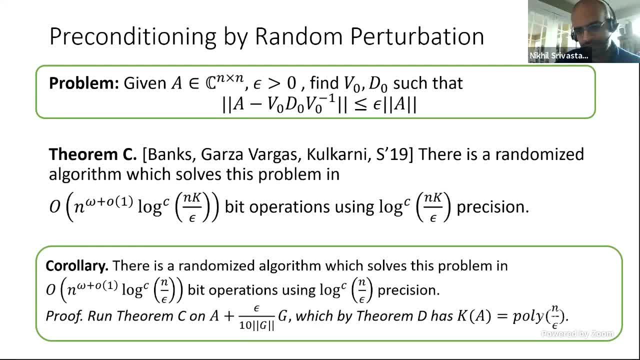 that you get a solution to this problem in time nearly matrix multiplication time. The algorithm is: you just take the matrix, add a Gaussian perturbation That makes this K of A condition number polynomial, And then you just run the theorem C algorithm. 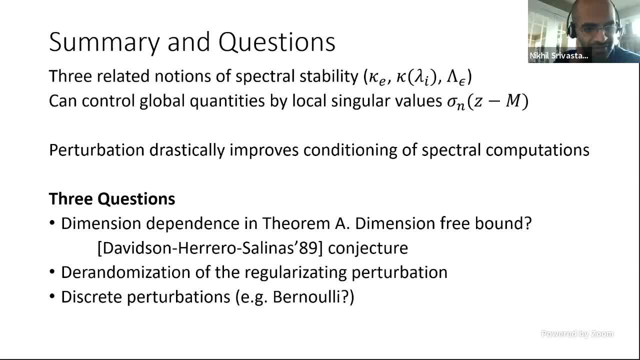 So OK, that's all I want to say. That's a summary of the talk. We use these three notions of spectral stability. The perturbation really improved the conditioning of these spectral computations, And there are several open questions. One is the dimension dependence. 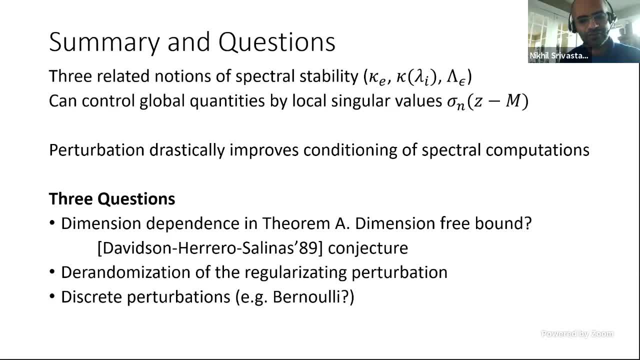 A really intriguing one is: can you de-randomize this? I have no idea how to de-randomize this. I still don't know how to find a perturbation E with these properties without using randomness. So anyway, that's it. Any questions? 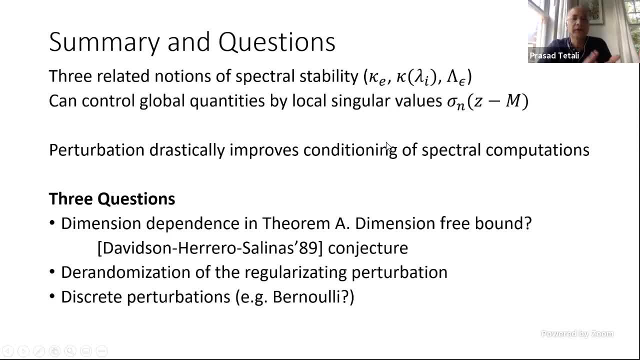 OK, great, Thank you, Nikolai. So people have questions. We are out of time, but we have a long break, So if people have questions, please go ahead. I have a question, So I was actually curious about the last part. 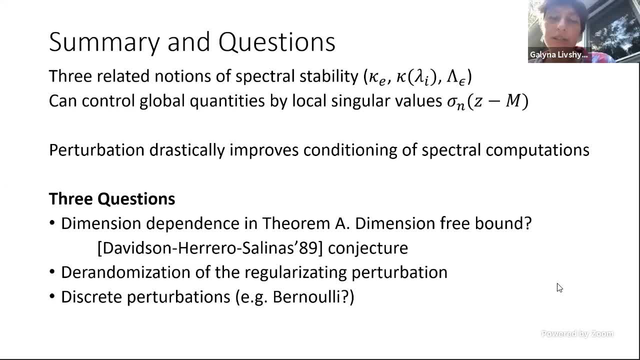 that you wrote the very last sentence that you wrote about Bernoulli. Do you actually expect it to be better, Or do you expect that the Gaussian will actually give you the best, Absolute best? I'm not sure. Algorithm estimate for regularization. 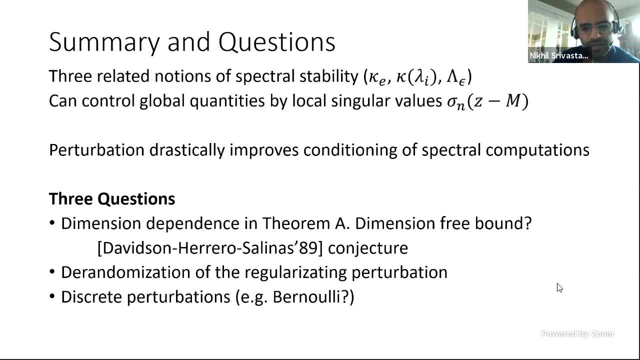 I don't expect the Bernoulli to be better. I don't have any mechanism in mind that would make the Bernoulli better. The Bernoulli is sort of a first step towards maybe being able to analyze sparse, random matrices which would have applications. 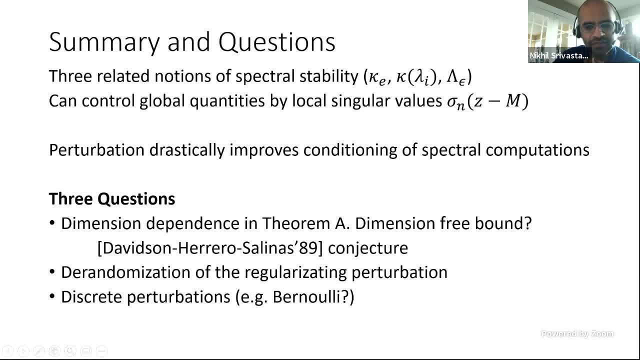 So it's mostly a technical challenge, Like all the arguments. OK, at least the arguments I presented in our papers use these limiting arguments. as epsilon goes to zero, That breaks for Bernoulli, The paper of Jan Sai and Sonny I. 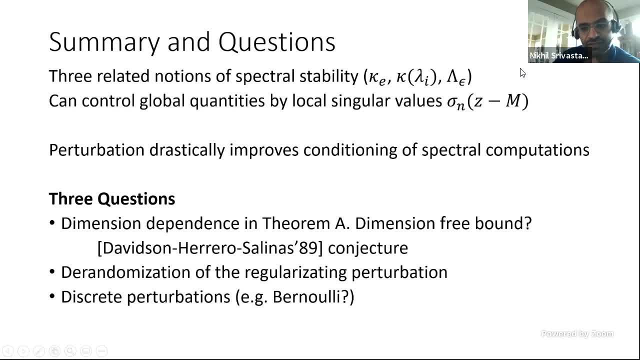 think might be more amenable to doing something with that, because they don't actually take a limit. They just set epsilon to be like 2 to the minus n or something. But there is some bottleneck in the current techniques that really requires epsilon. 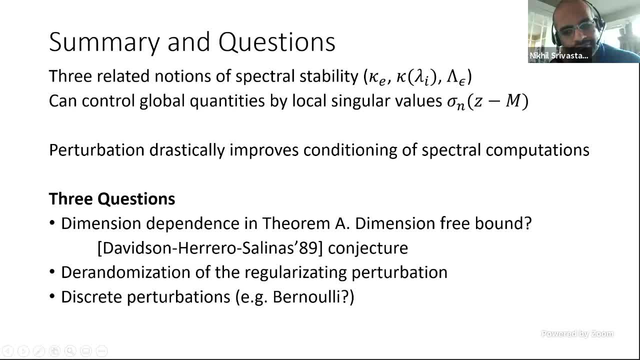 It requires absolutely continuous density, So I'd like to really want to understand whether that's really needed. Any other questions? Yeah, like you were just talking about this Spielmann and Tang result that you used In a recent archive paper, people are looking at what happens if you add sparse Gaussian noise. 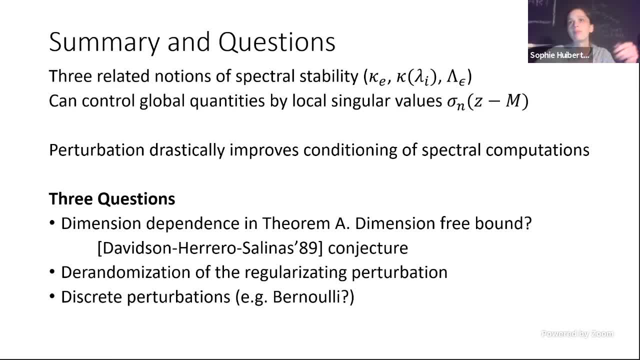 Do you think that your result is going to be better? Do you think that your results could like, basically use this and extend to that case as well, where you have sparse noise Or like low rank noise? Yeah, so it's very possible. 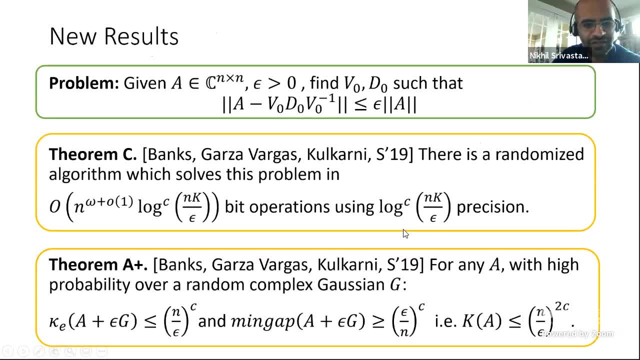 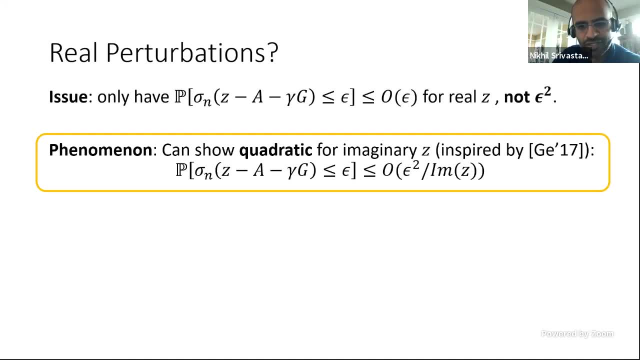 I mean, the key thing you need at a technical level to prove this kind of result by this technique is you need a tail estimate with a correct dependence on epsilon. So you need to prove that this probability. so let's do complex for now. 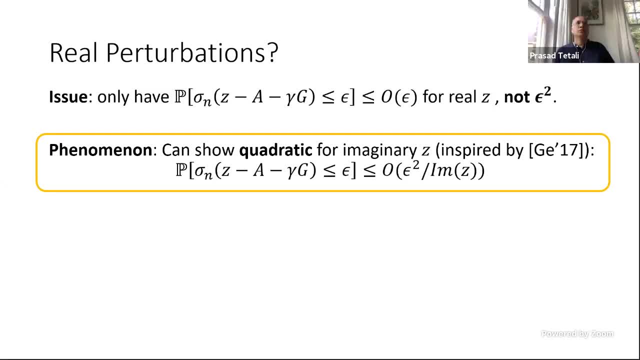 You need to prove that this probability is less than epsilon squared, because you need to take this limit divided by epsilon squared. So if you can do that for, let's say, sparse Gaussian, then I mean, yeah, that's the technical problem. 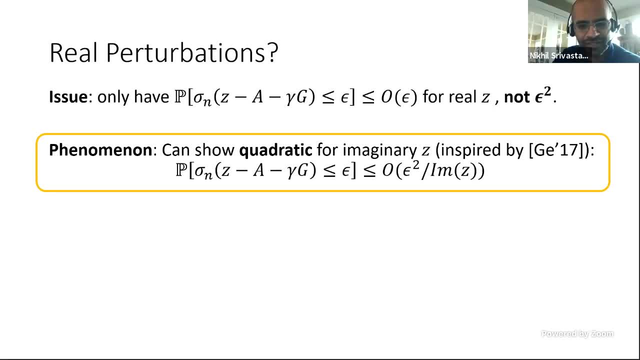 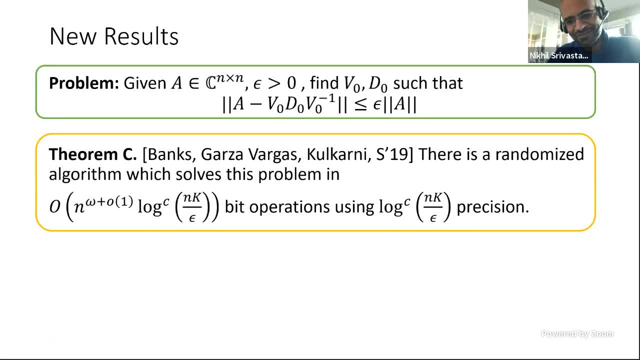 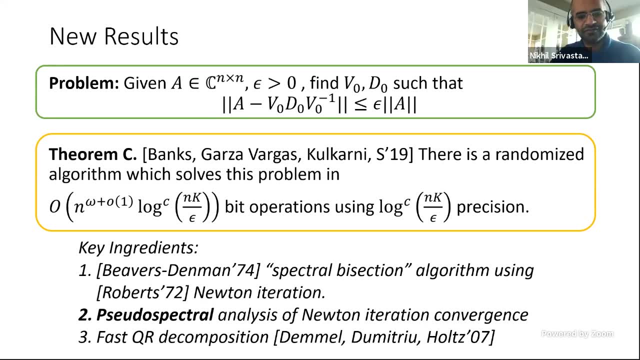 So I didn't tell you what theorem C is, what the algorithm is. So it's an algorithm called spectral bisection. It's a divide and conquer algorithm which works by recursively computing spectral projectors onto subspaces that account for roughly half the spectrum. 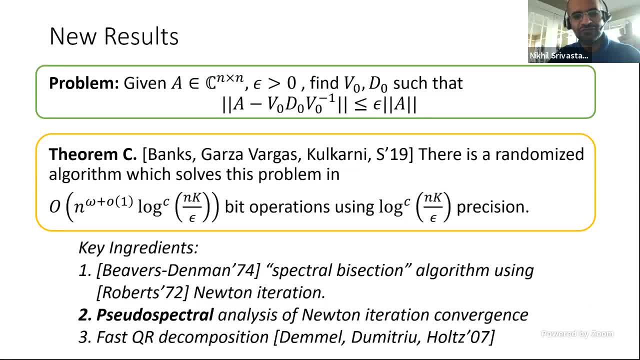 Now to do that, one thing you need to do is you need to find a line in the complex plane that divides the eigenvalues roughly in half, And the randomness is only used in that, So I'm pretty sure you can de-randomize it.